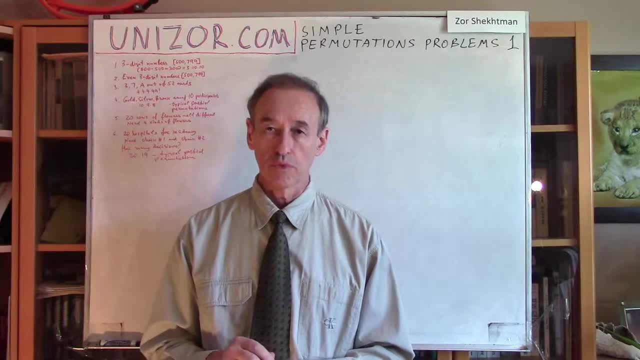 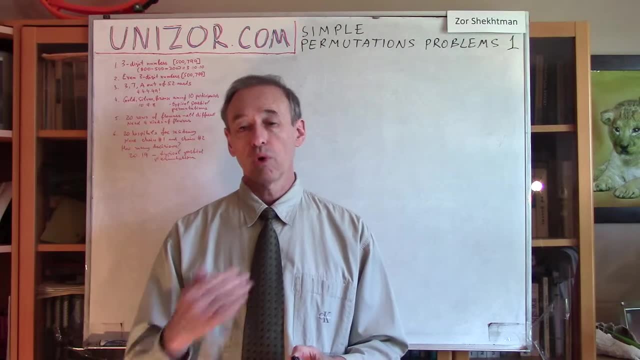 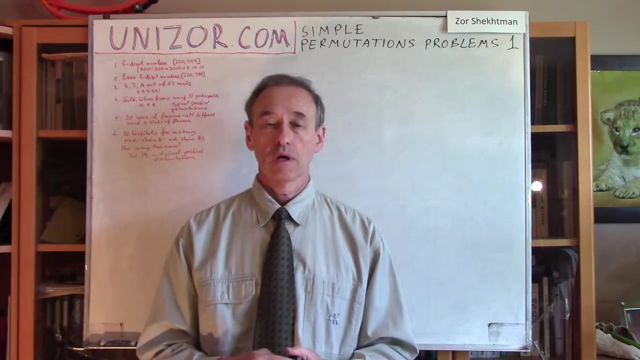 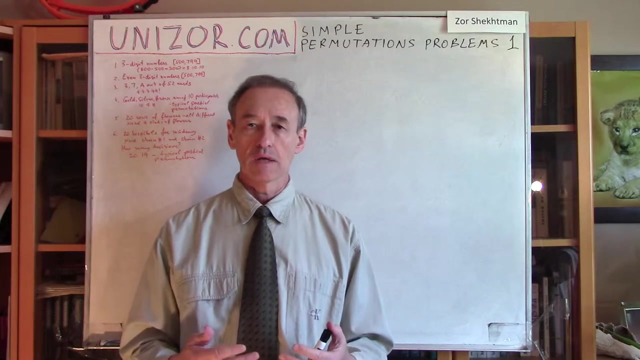 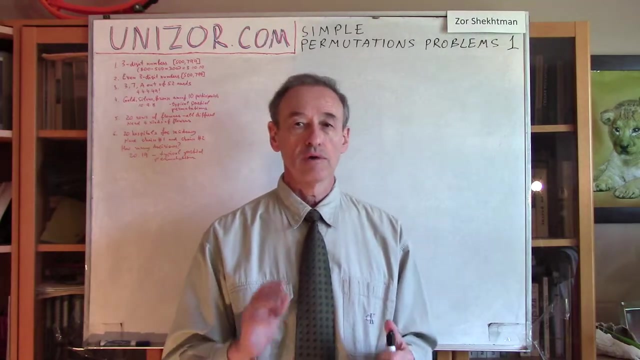 And I recommend you to try to solve all these problems just yourself. Don't read the solution, Which is also presented, But only after that it makes sense actually to listen again to the lecture. Compare your solution to whatever I'm presenting here, Because the whole thing is actually aimed as a tool to develop your logic. So this is all about logic. Combinatorics is very logical thing. 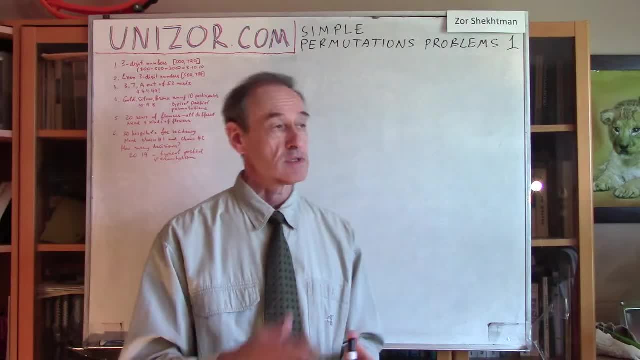 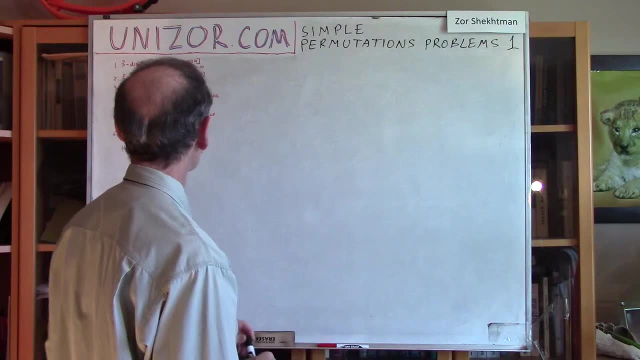 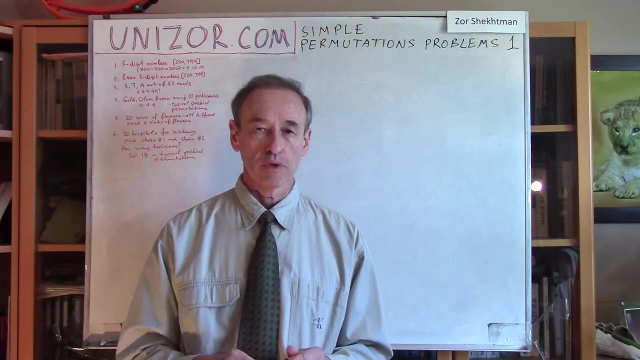 So I recommend you to do it yourself first and then go to the lecture. All right, So let's just do one by one. I have six problems to discuss. They are really simple, So yes, And one more statement which I would like to make. 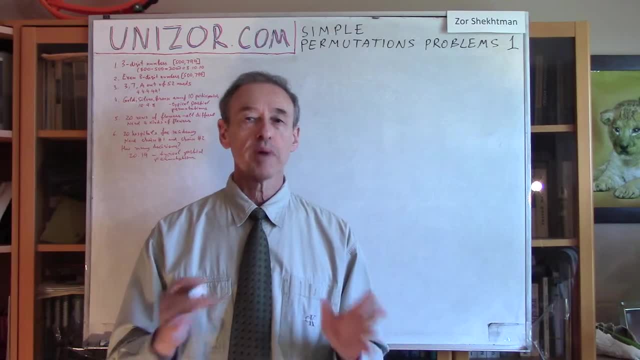 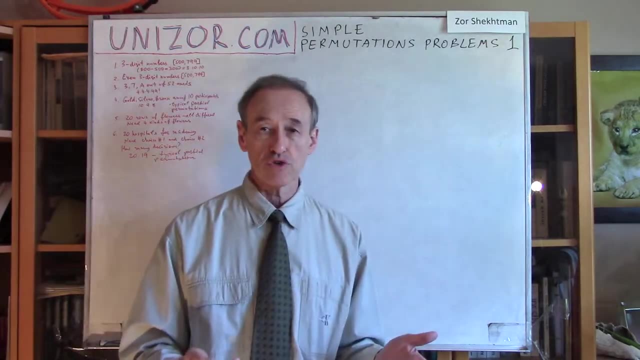 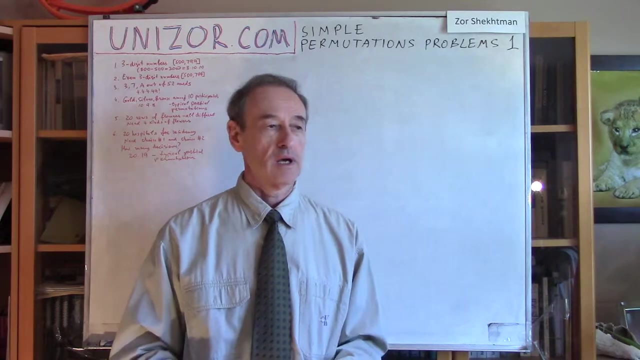 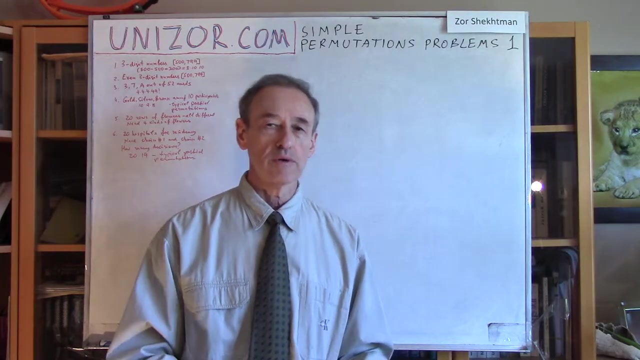 Don't try to remember the formulas of the combinatorics. Probably the only formula which you really might remember is the number of permutation of n different objects is n factorial. It's simple, It's like it goes immediately Into your mind. But everything else- the number of combinations with repetition, without repetitions, all logically derived from this. 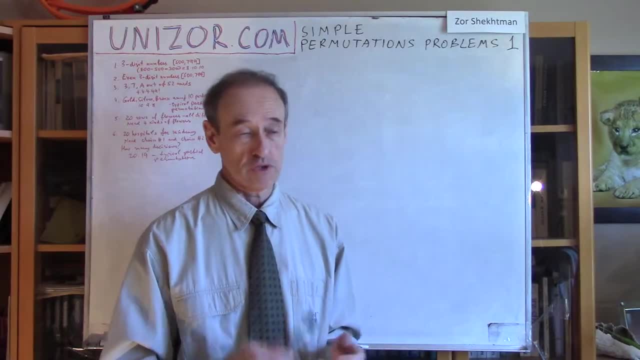 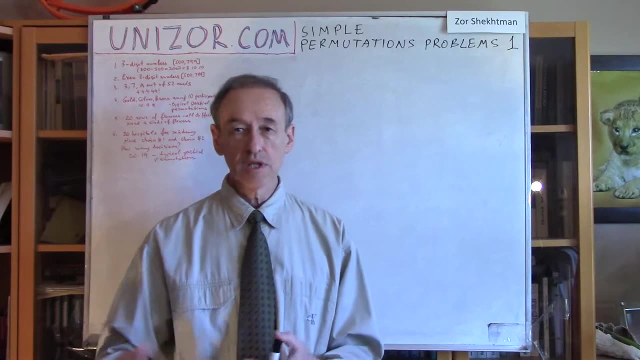 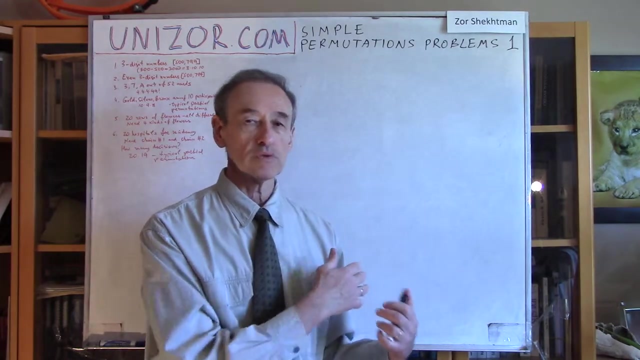 From this one and only formula about number of permutations, which is n factorial. So what you have to remember is not the formula, but the logic which leads to any formula of the combinatorics. So that's very important And that's why I'm not really using any formulas. 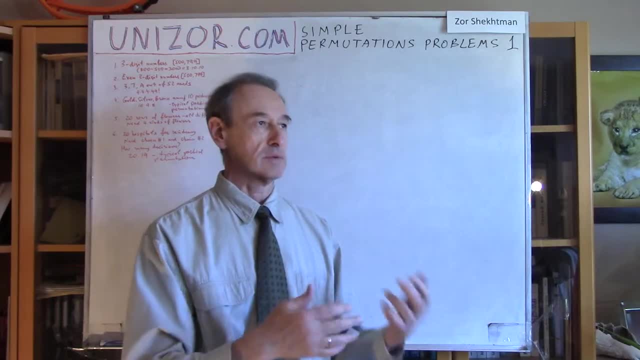 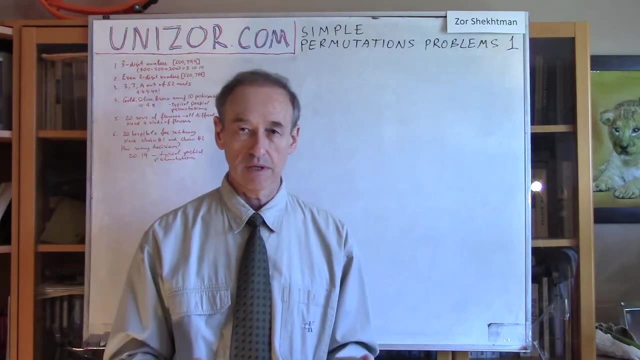 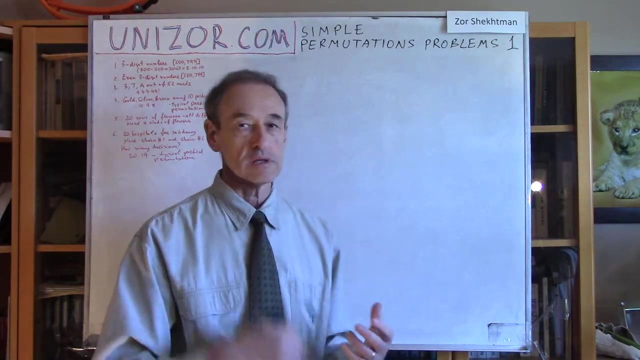 I'm not using any formula here, like calculate how many different combinations from five by two or something like this. I'm not asking about all these calculations of the formulas. What I am presenting is logic behind the solution, And that's very important. So forget the formulas. Now three digits numbers. Okay, How many different three digits numbers? Two digit numbers are between 500 and 799.. Inclusive, So both n's are included, Alright. Well, let's just think about it. All these numbers start with either 5 or 6 or 7.. 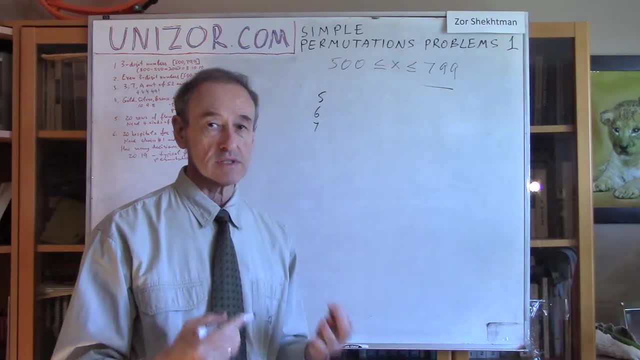 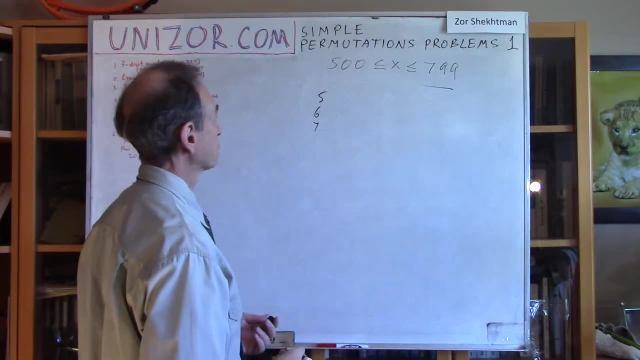 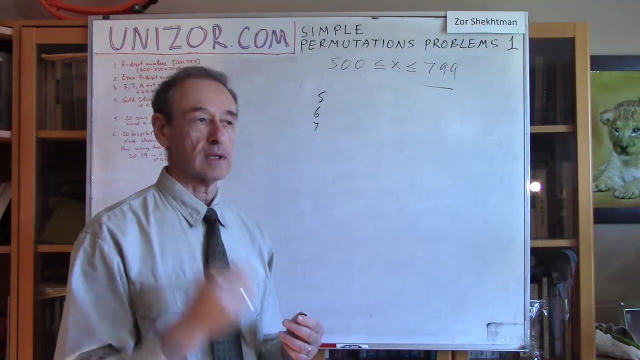 So For the choice of the first digit Of our three digit number, We have three different choices. Now Everything else actually is not fixed, Which means any other place can have any other digit, 00 or 53 or 99 or whatever it is. 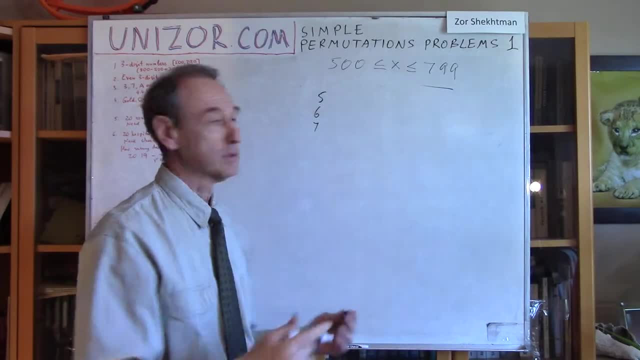 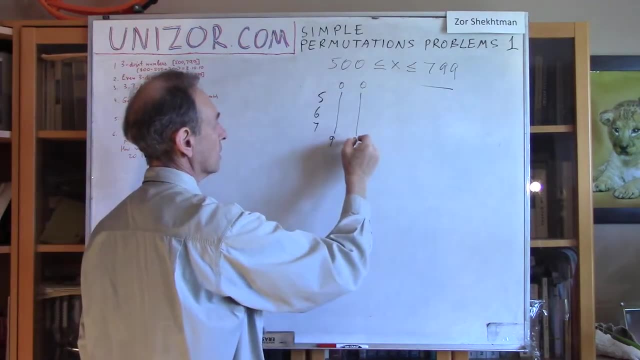 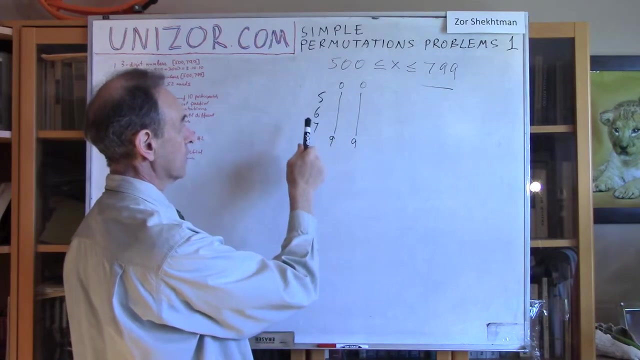 So all other combinations are valid. And how many combinations we have? We have from 0 to 9 as the second digit And from 0 to 9 as the third digit. So our choice is among all these numbers, Which have three choices. for the first digit, 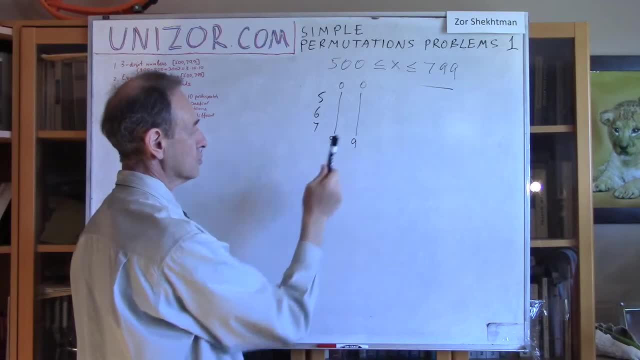 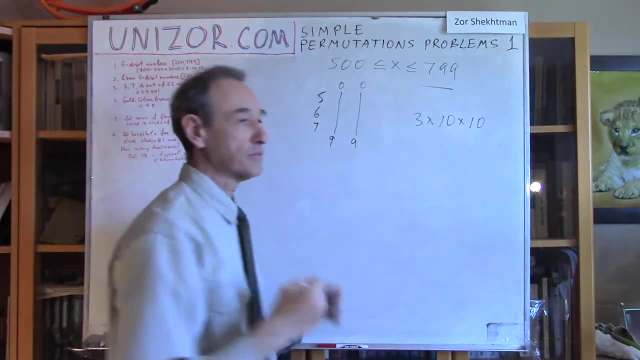 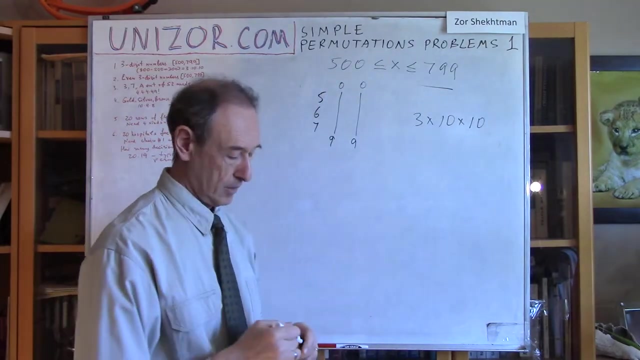 Ten choices for the second And ten choices for the third. So all together it makes 3 times 10 times 10.. Different choices, Different three digit numbers, Which are among these. Well, You can obviously say that It's very simple to calculate. 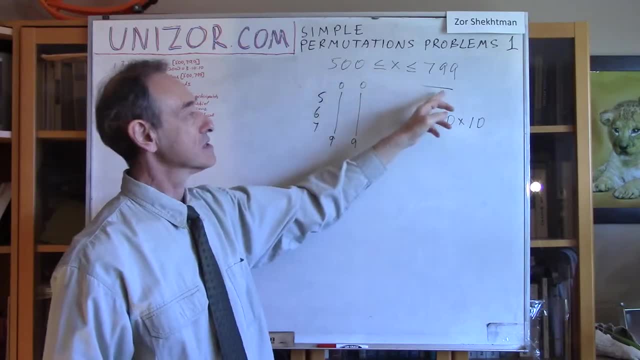 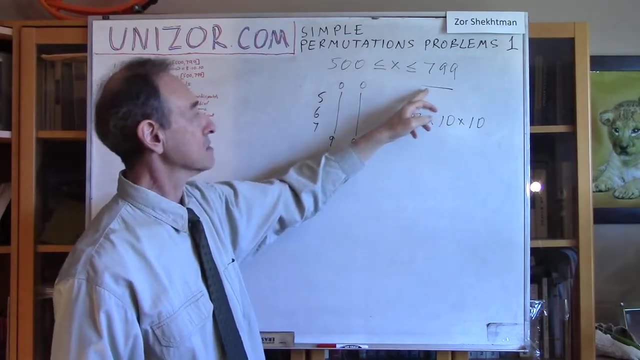 Because if you need all the numbers between this and this, You have to subtract from 800- 500. Because this is inclusive on both ends. So you have to subtract from 500- 800. And you will get 300. Which is exactly the same as this one. 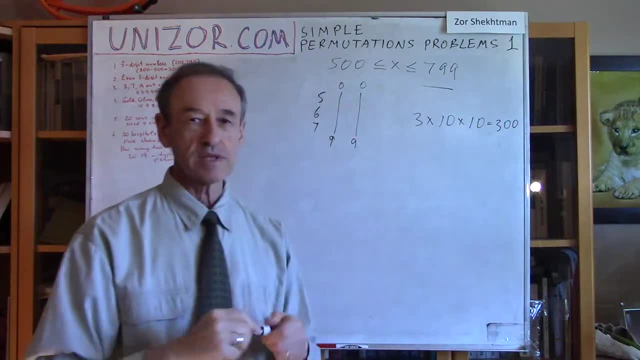 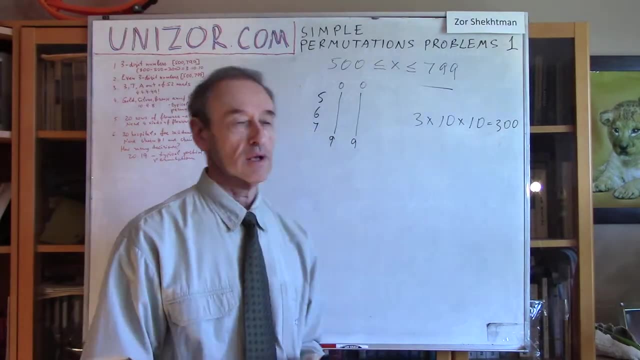 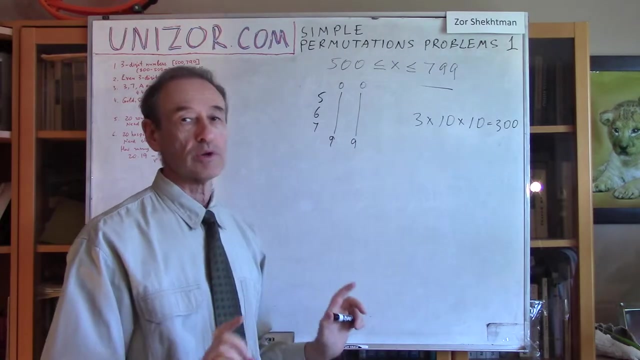 Yes, Obviously you are right, And the purpose of this particular problem Was not derivation of the number 300. Which is kind of obvious From the subtraction thing, But to present the logic, How to derive it combinatorically. And that was the only purpose of this problem. 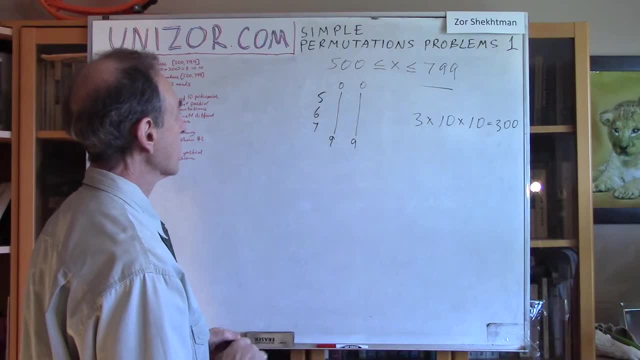 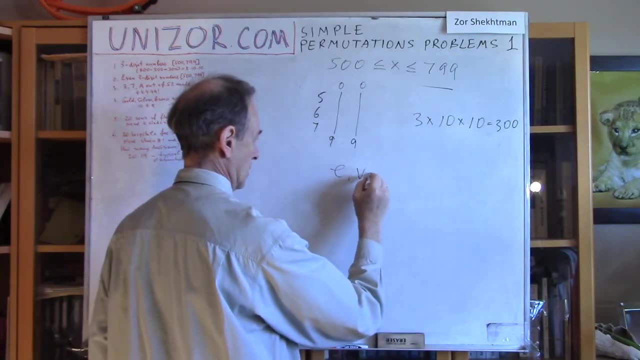 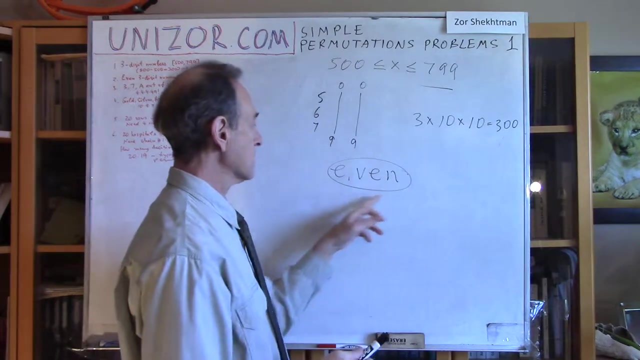 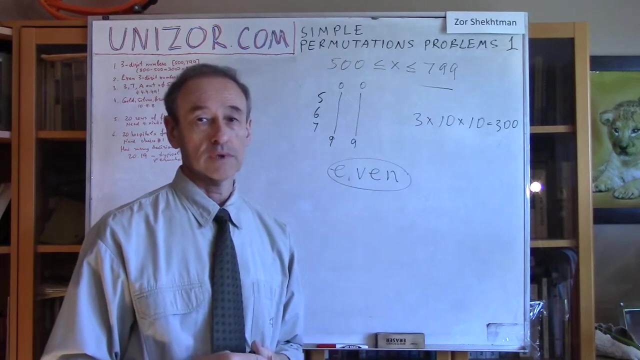 Okay, Now The second problem. Exactly the same problem, But I'm interested only in even numbers. Again, From the general considerations You can say that the even numbers Are basically half Of whatever we have here, Right? So if all together I have 300. 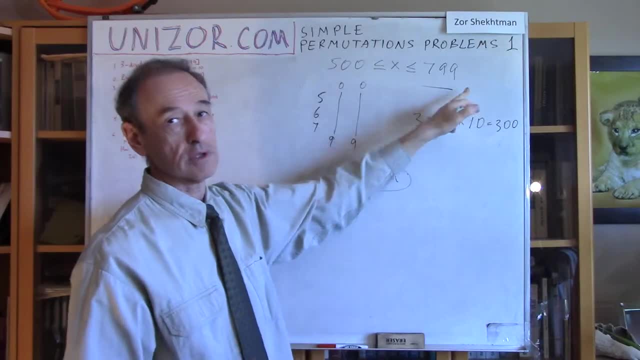 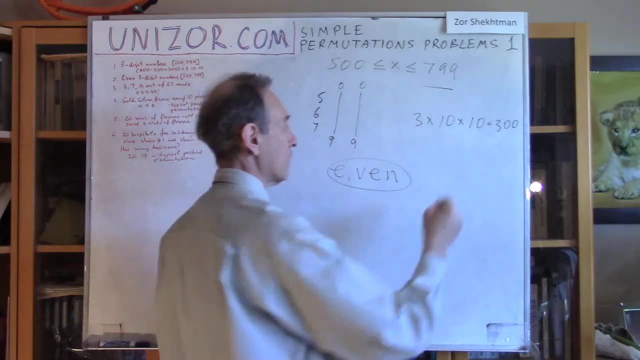 The first one is even, The last one is odd. So basically we can break them into pairs And each pair contains even odd, Even odd. So half of this, It's supposed to be 150.. Right, Half of the 300.. 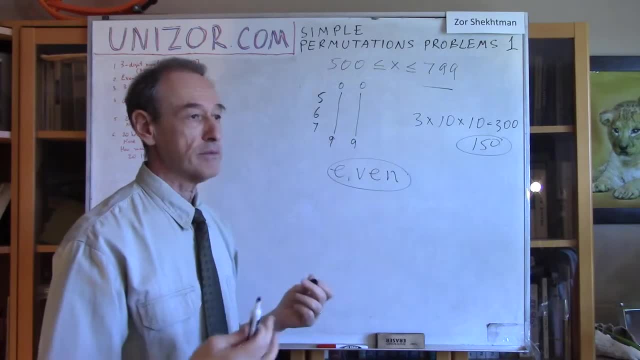 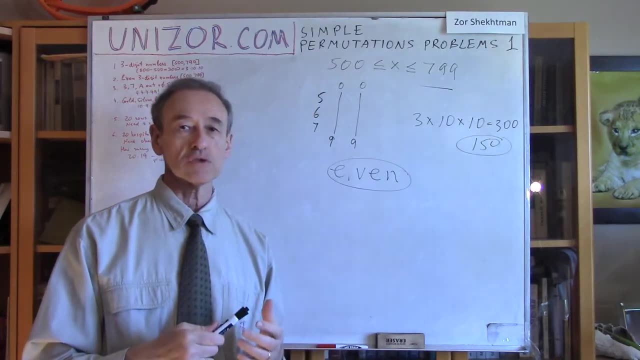 But let's check if we can Derive this particular Number Combinatorically. Now, What is The main characterization of the even number? Well, It's the last digit Which is supposed to be even, Right. So 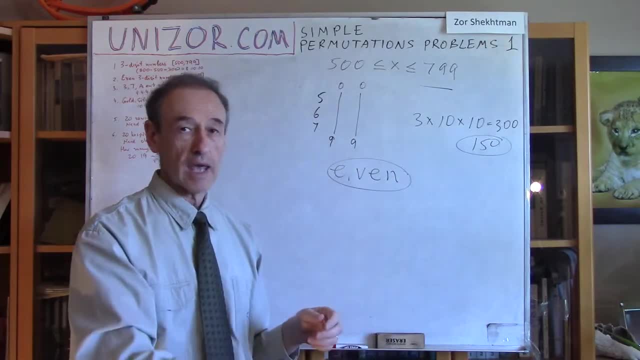 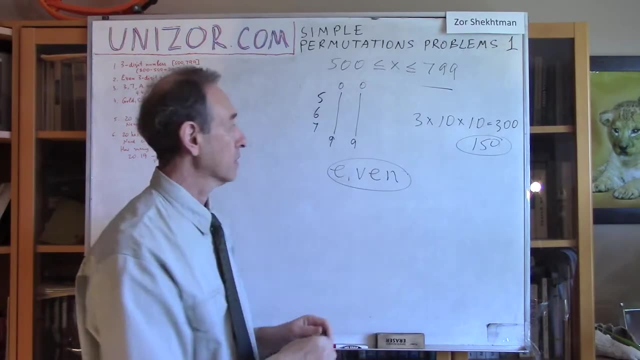 If the number ends with 0. Or 2. Or 4. Or 6. Or 8. It's even- I'm talking about- only The last digit. Everything else Is really irrelevant. Right, So For. 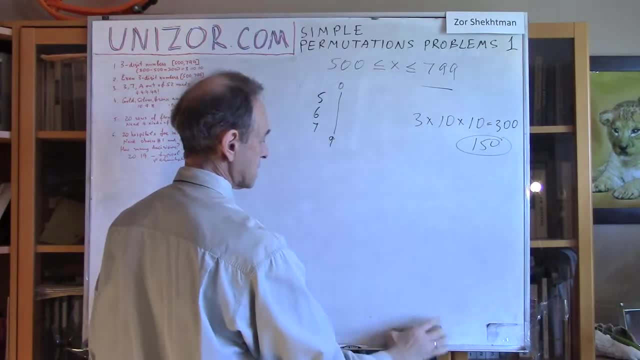 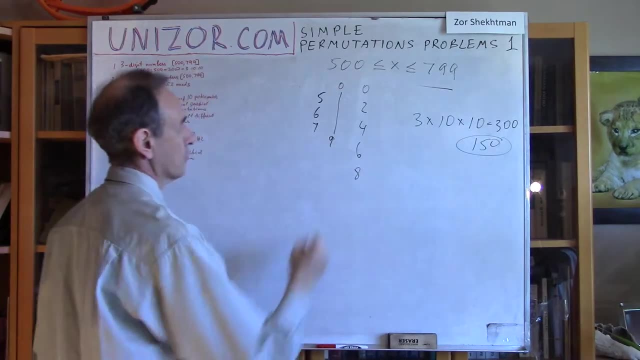 The third Digit We have In case We're looking for Even number: 0., 2., 4., 6. And 8. Which is 5 different choices, Which means In here I have to have. 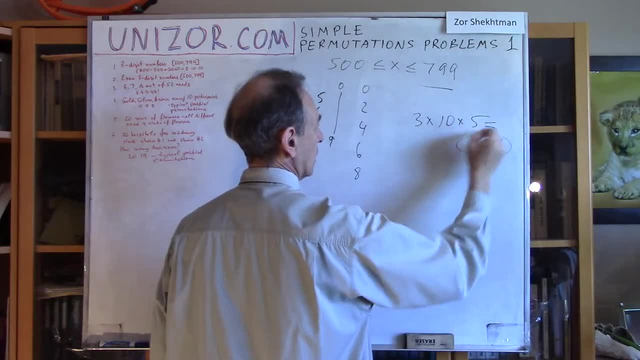 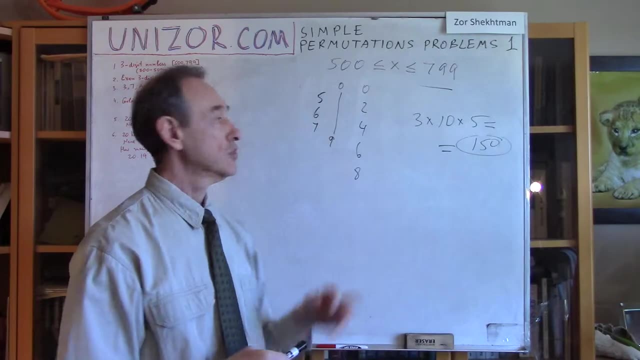 By 5. Which is Obviously Equal to 150.. So We can derive Exactly The same 150.. Using A Purely Combinatorial Considerations, 3 choices For the first Digit: 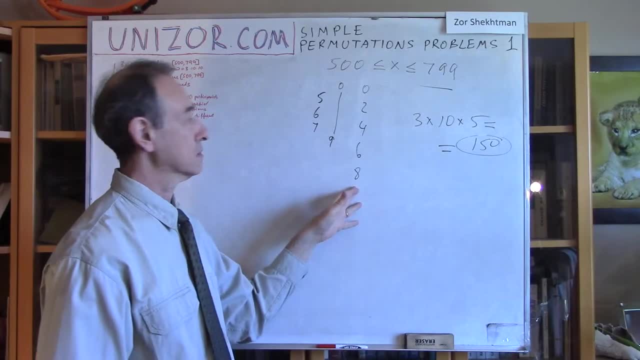 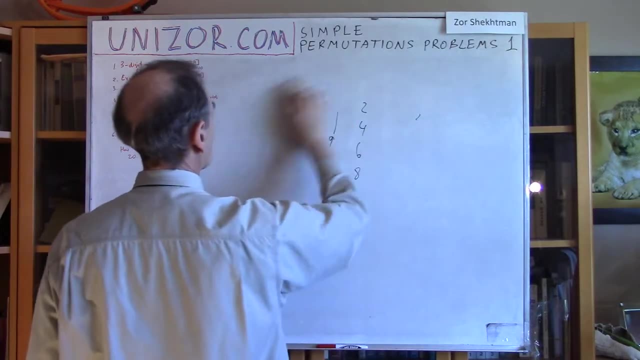 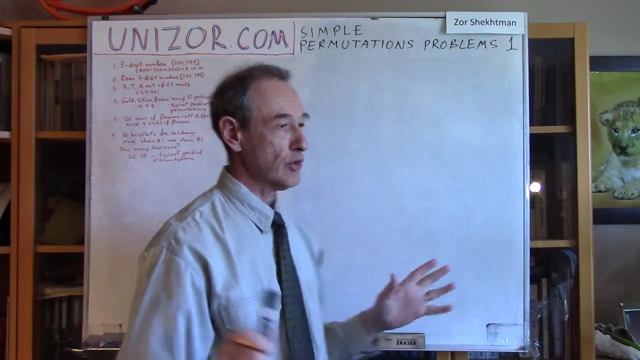 10 choices For the second And 5 choices For the last. The third Digit And we get 150.. All right, That's the second Problem. Let's move on. Third Problem: Okay, Let's consider. 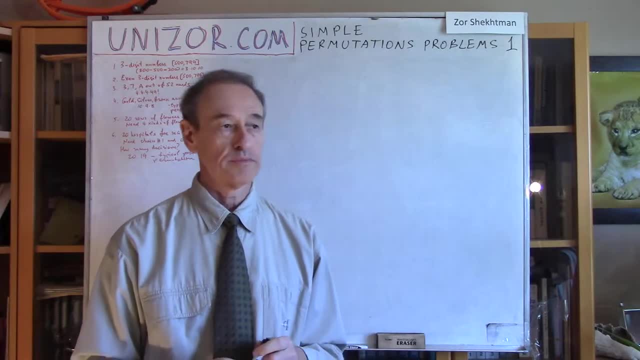 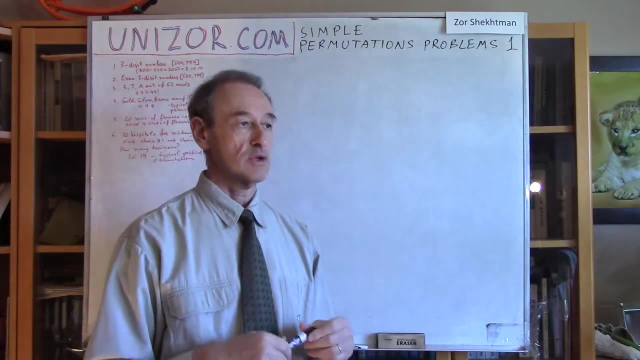 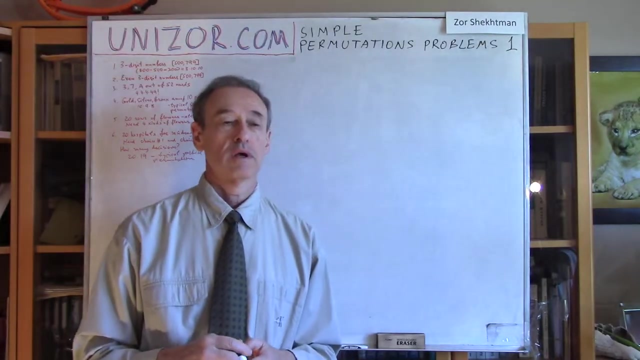 You have 52. Cards- Regular Deck Of Cards. Now, Well, Let's say You are Poker player, Which means, Well, There is A famous Literally Work Which is Called. 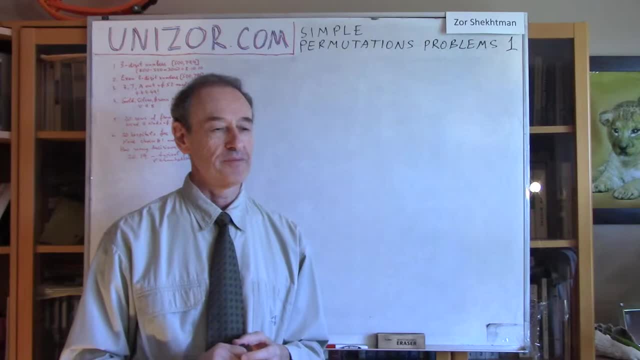 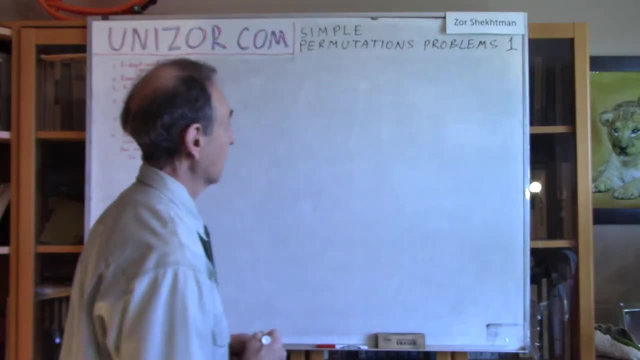 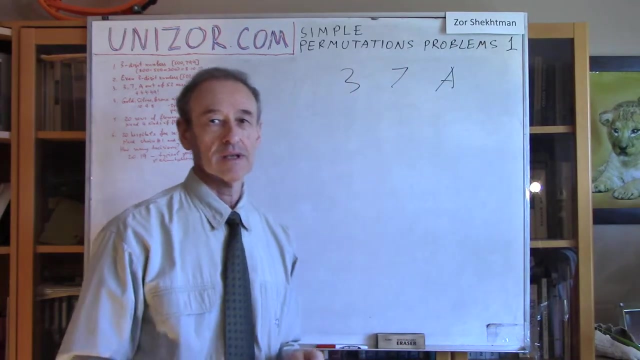 The Queen Of Spades In Russian Literature. And So There Was Guy, A Gambler, Who Was Looking For A Combination 3., 7. And Ace. 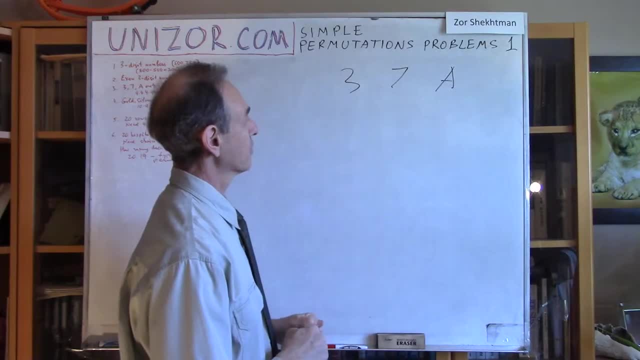 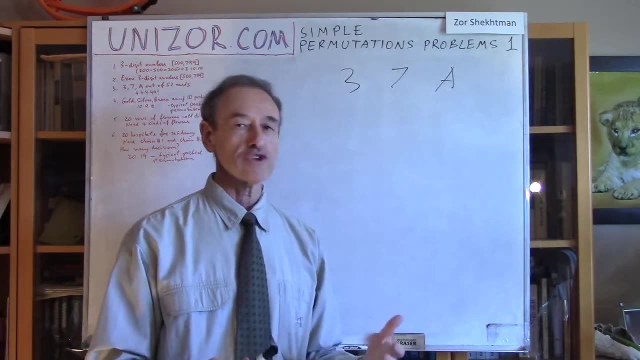 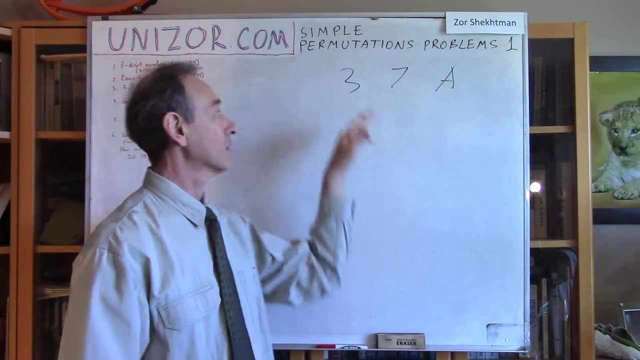 My Question Is: Let's Say, We Shuffle The Cards And Then The First Three Cards Are 3., 7. And Ace, In This Particular Order. 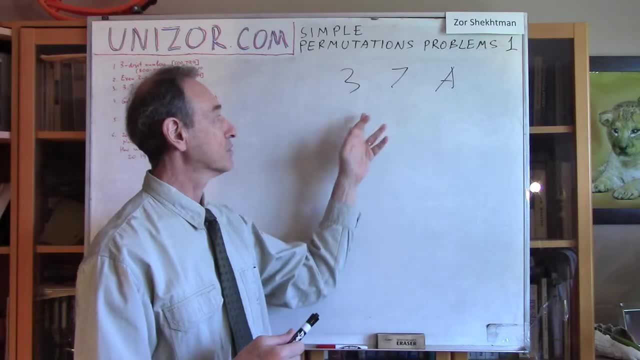 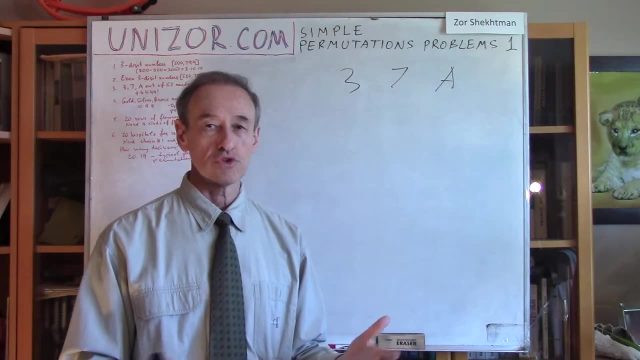 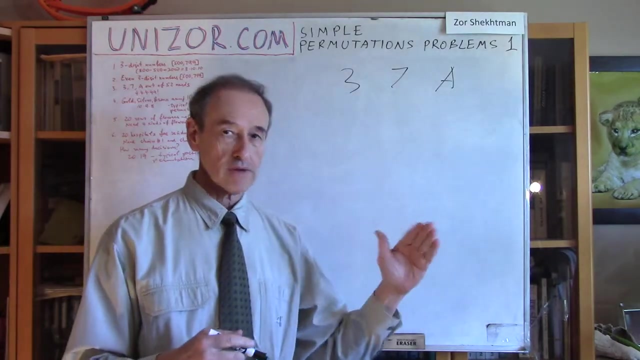 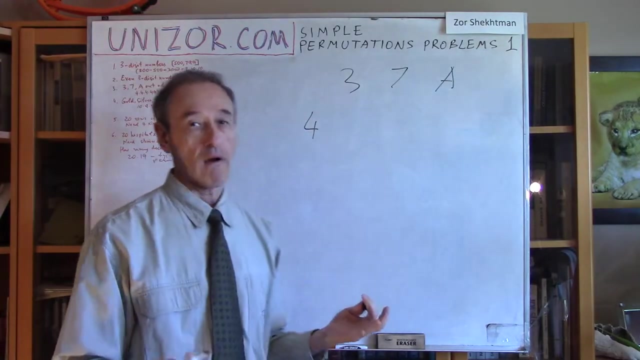 My. So The 3., 7. And Ace, As The First Three Cards In This Order, Exists When You Shuffle The Cards, When You Shuffle The. 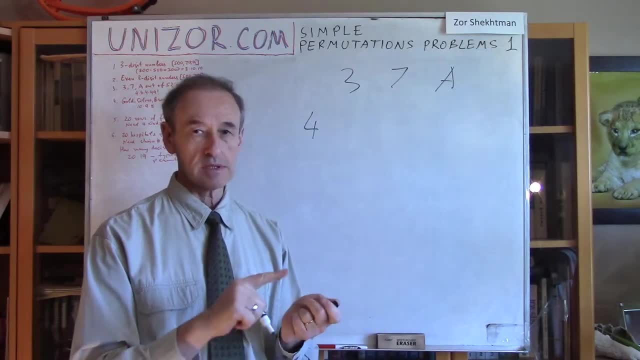 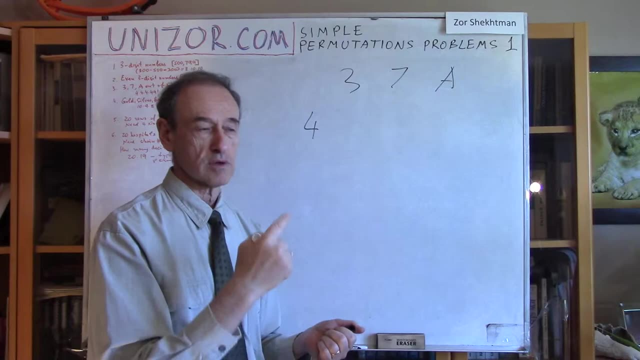 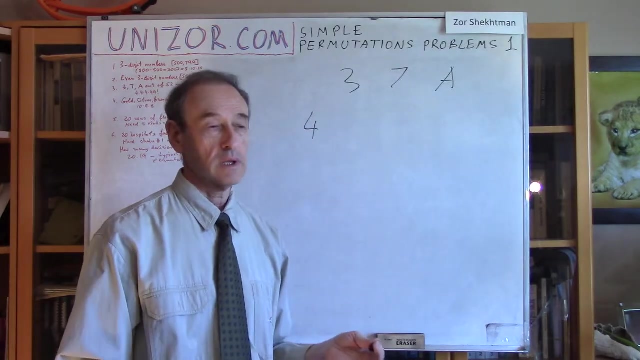 Deck Of Cards. Well, Let's Just Think: Four Different Trees, Three Of Hearts, Three Of Spades, Etc. Now Next Is I Need The Seven. 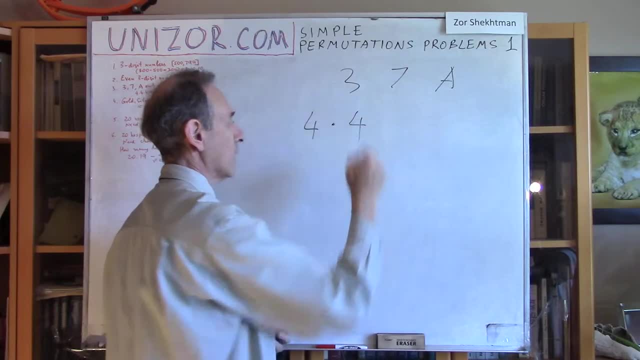 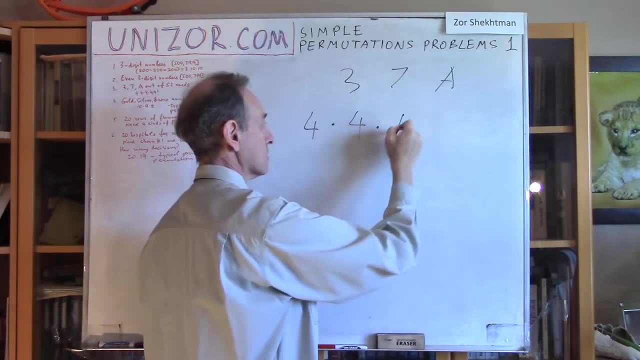 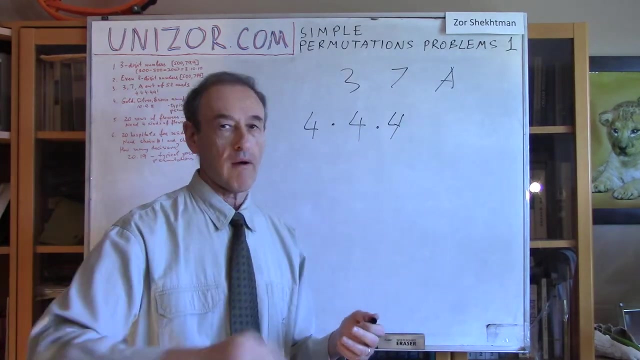 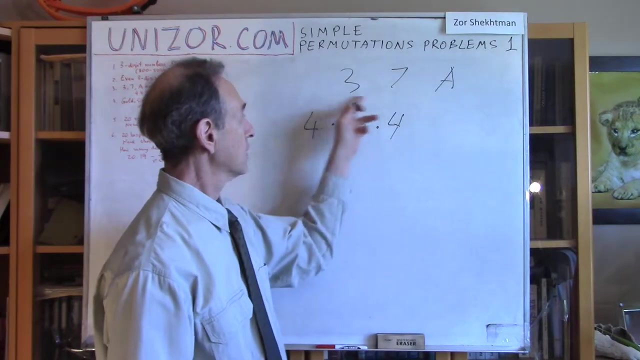 And There Are Also Four, Seven, Again Seven Of Clubs Of Diamonds, Because Again There Are Four Different Aces. Now All Other Cards Can Be. 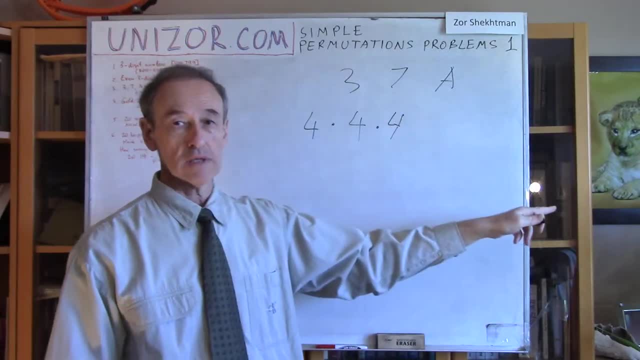 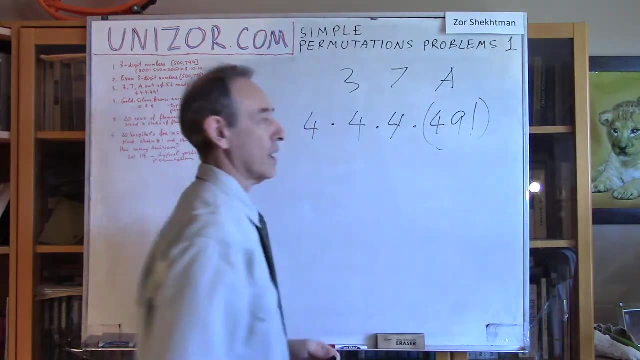 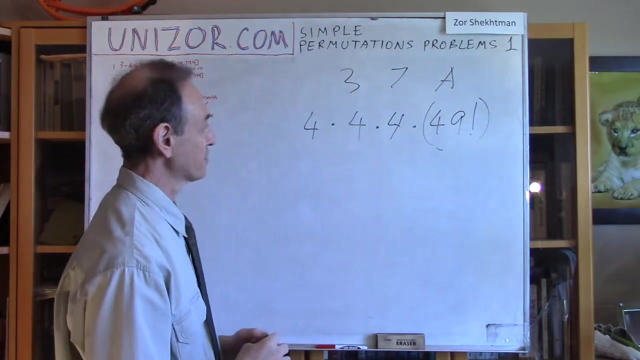 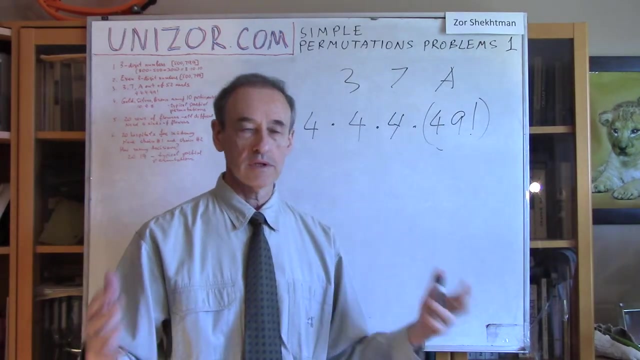 In Any Order. I Don't Really Care, And All These Permutations Of Other Cards, Now I Need To Remember. All Right, So The Total Number: 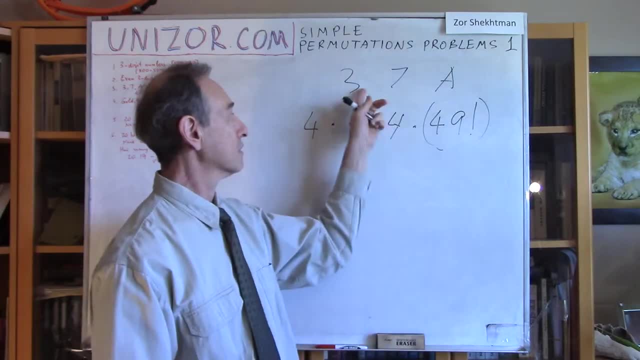 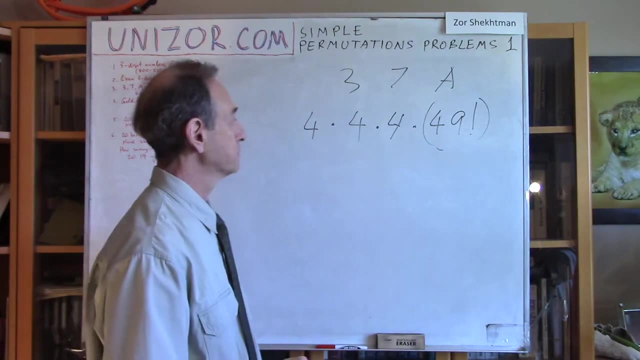 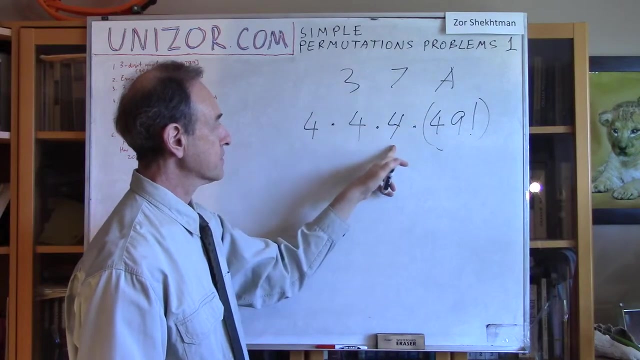 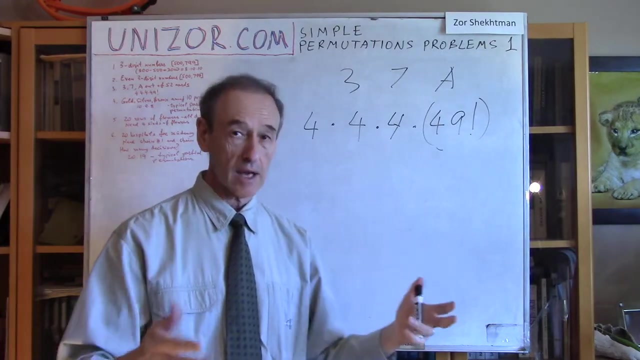 Of Different Different Card Decks. Actually, When The Top Three Are Three, Seven And Ace Are This Number? Whatever This Number, That's The Total Number. 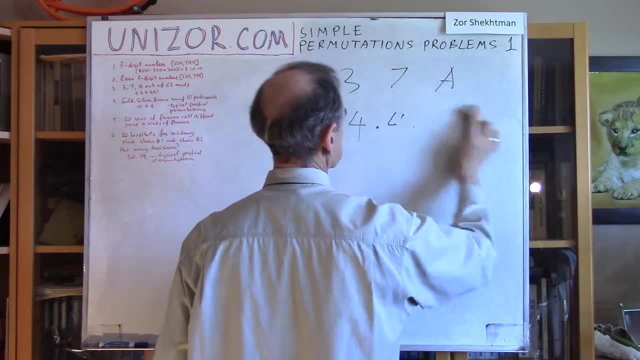 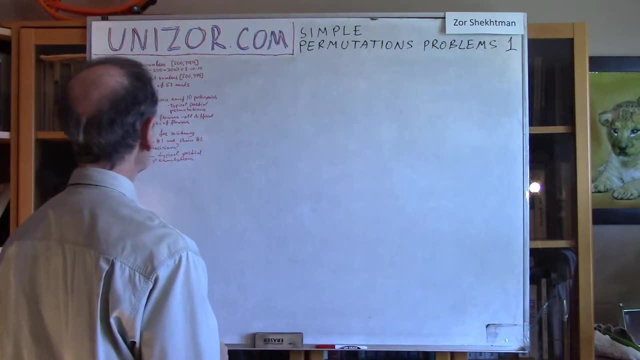 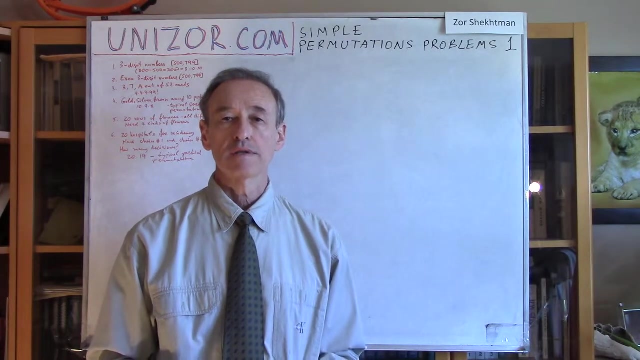 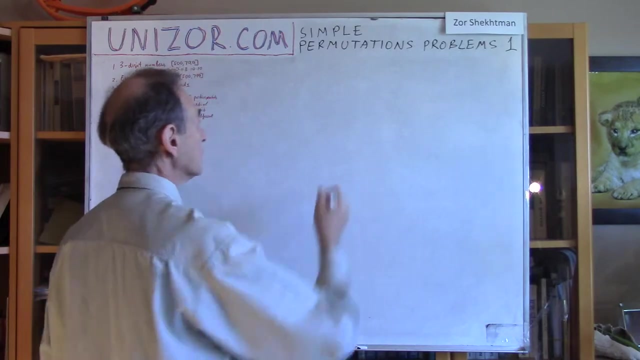 Of Different Permutations Of Deck When The First Three Cards Are Three, Seven And Ace. Next Problem. Next Problem: We Have Ten Participants In Some. 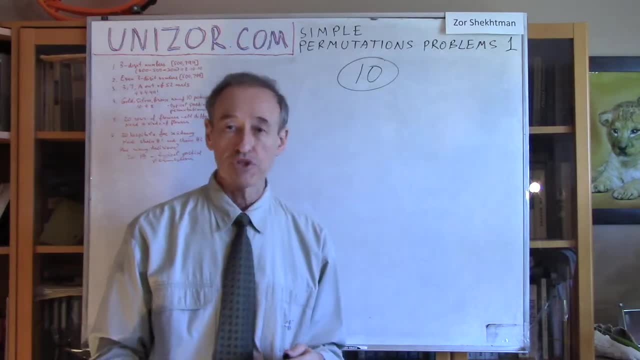 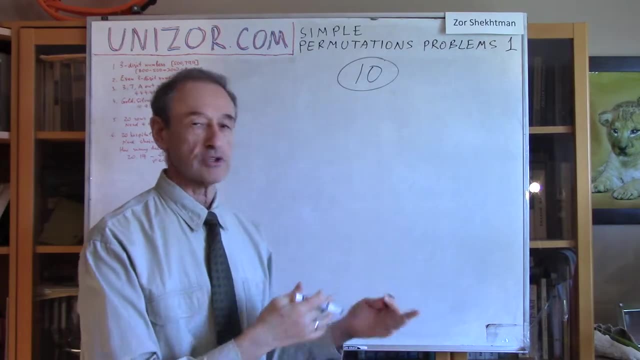 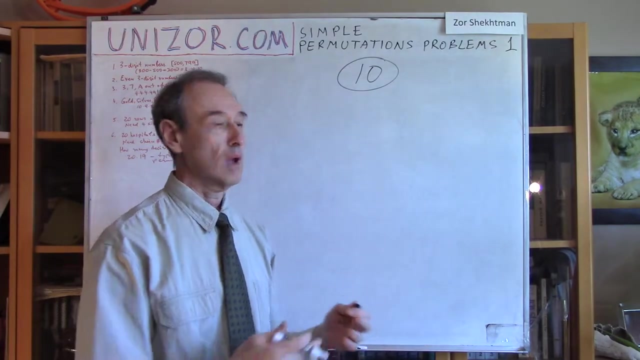 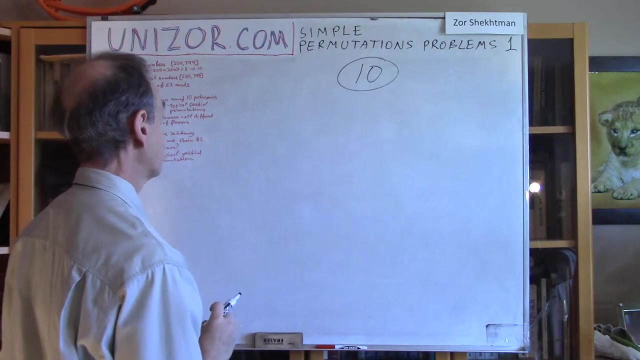 Of Ten Out Of Ten Different Participants In The Competition, Well, The Results Can Be Obviously Different. Different People Can Take Different Places. So My Question: 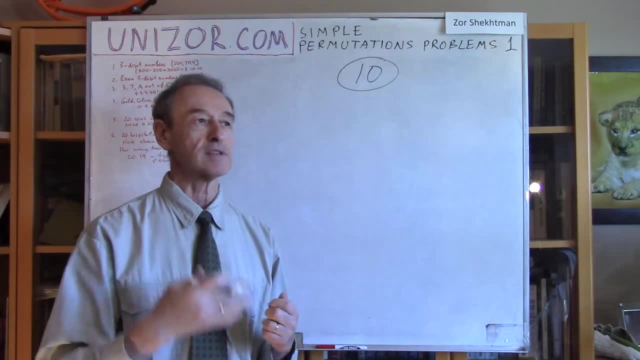 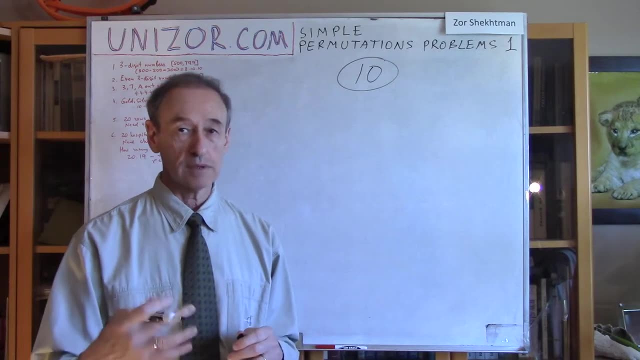 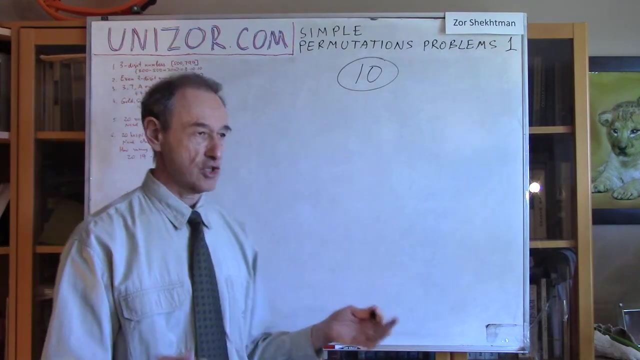 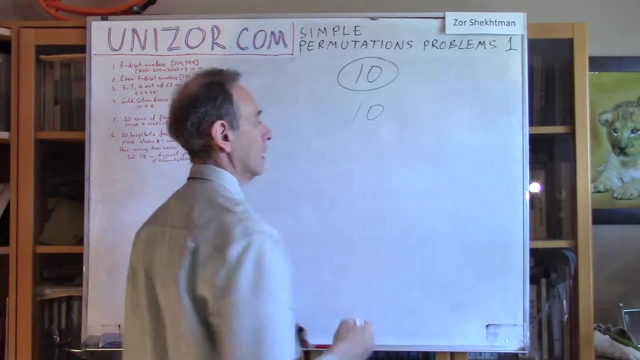 Is: How Many Different Results Of The Of The Metal Distribution. Let's Say, Yeah, That That's A Proper Right. How Many Different Metal Rest Distributions? 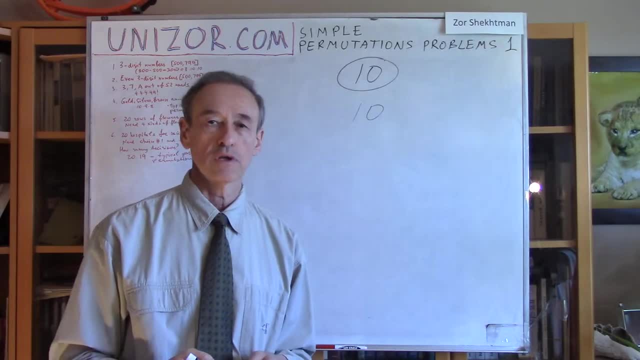 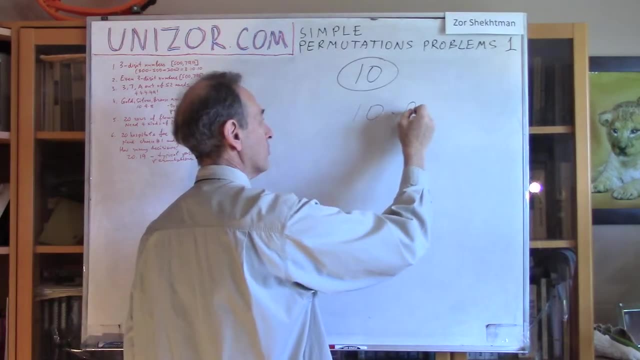 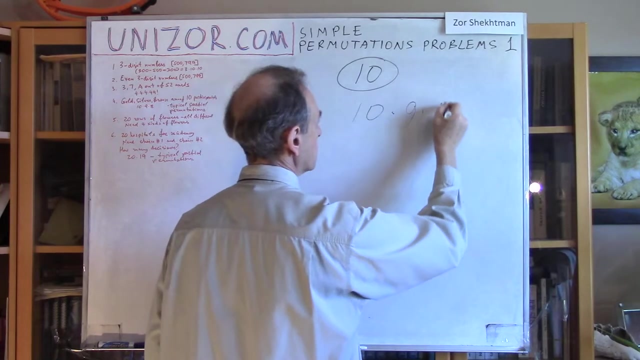 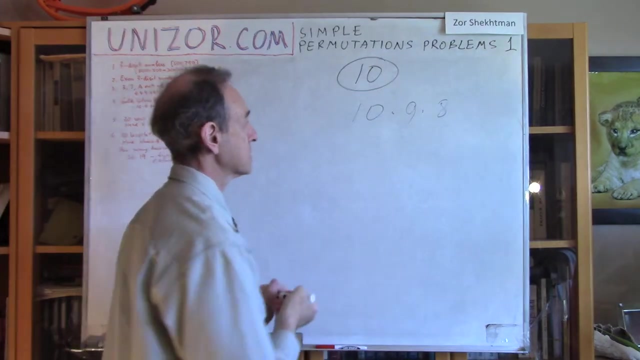 Among Ten People Exist Right. So Again, When The Gold Medal Is Chosen, There Is Only Nine Participants Which Can Get The Silver Medal, And 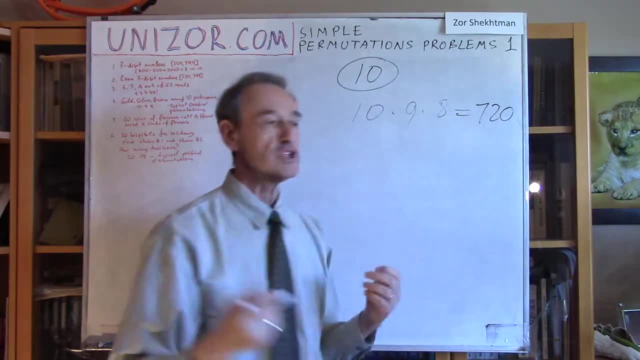 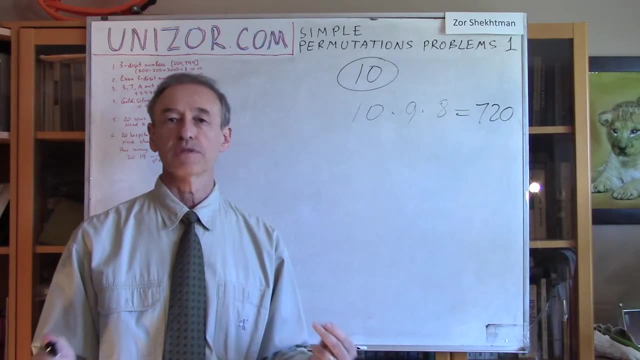 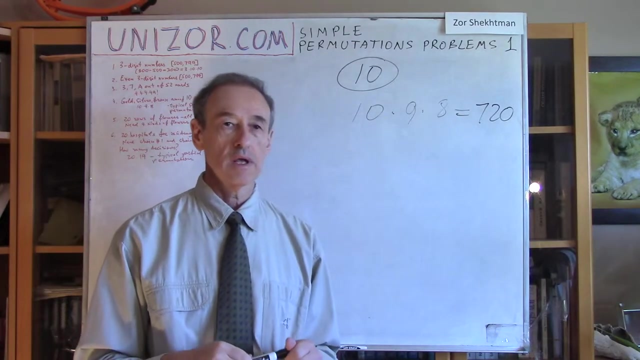 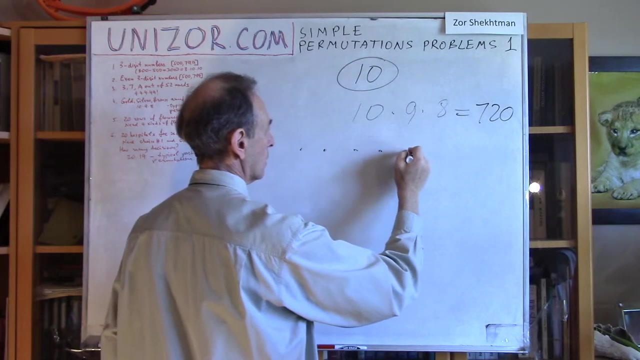 After Silver Medal Is Assigned. We Have Eight People To Get This. So Basically, You Can Envision It In The Following Model. Let's Say You: 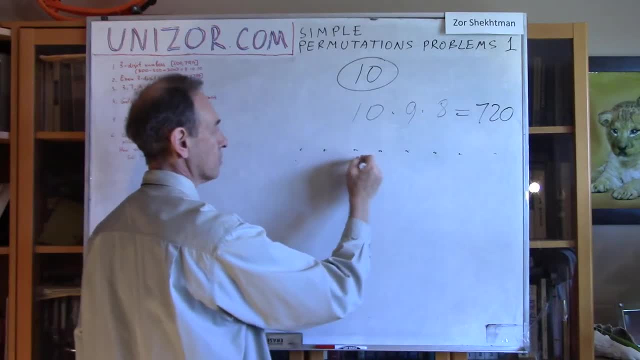 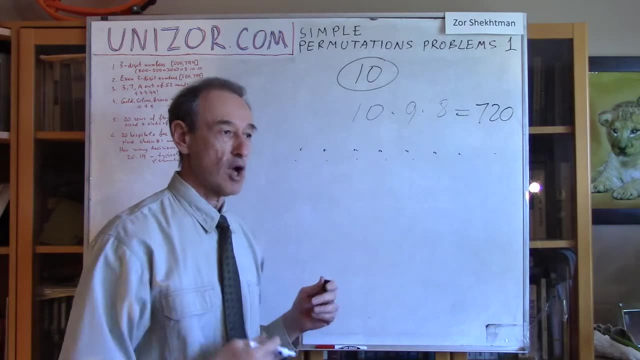 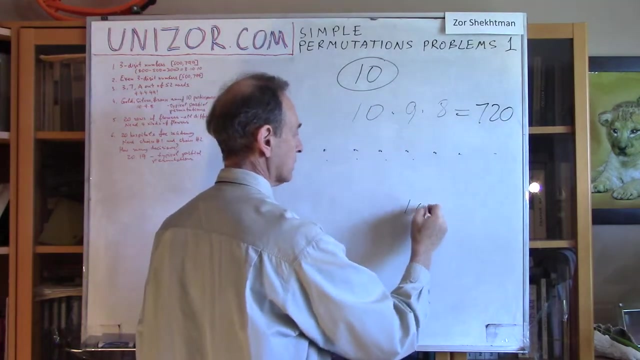 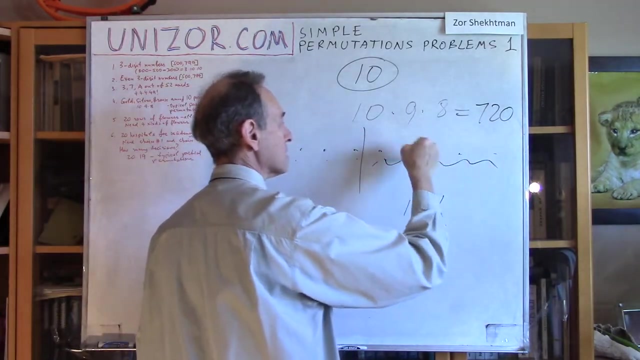 Have Ten Participants, So You Put Them Into Order: Number One, Number Two, Number Three, Number Ten People. Well, Obviously Ten Factorial Right Now. But 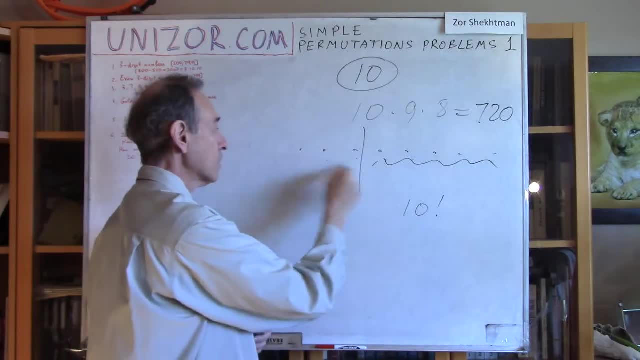 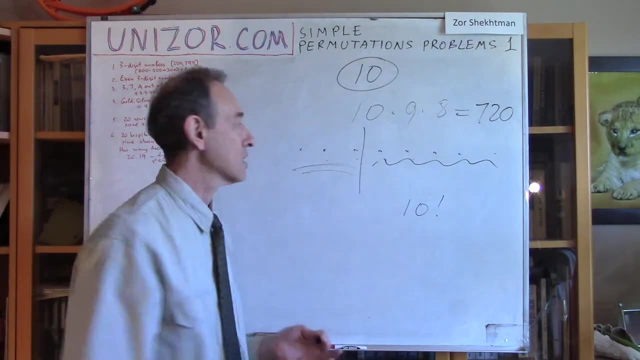 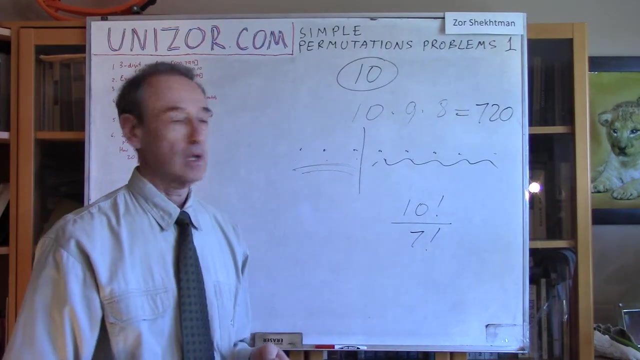 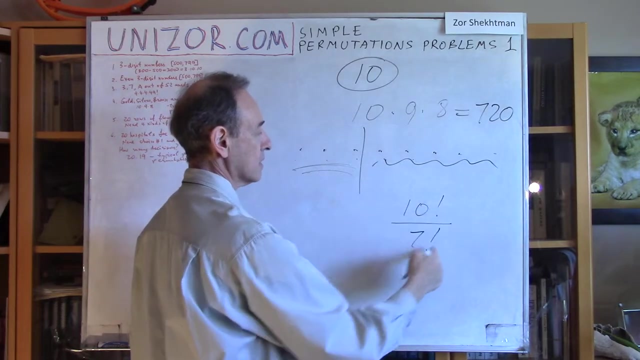 The First Three Are Fixed. So No Matter How These Guys Are Permuted, The First Three Will Have Exactly The, Because Ten Factorial Is The. 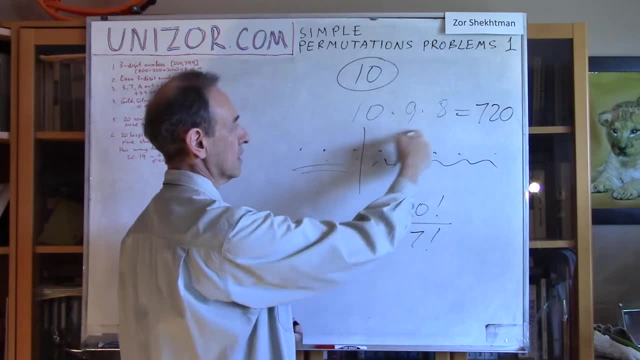 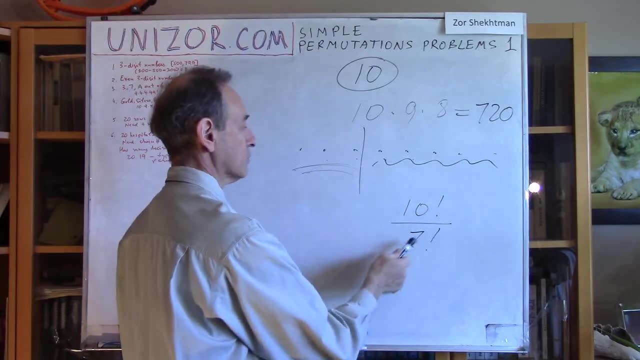 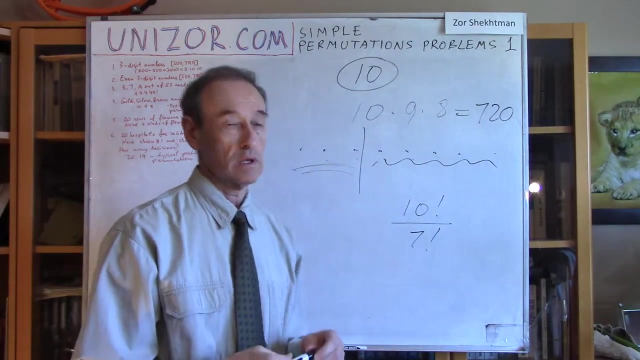 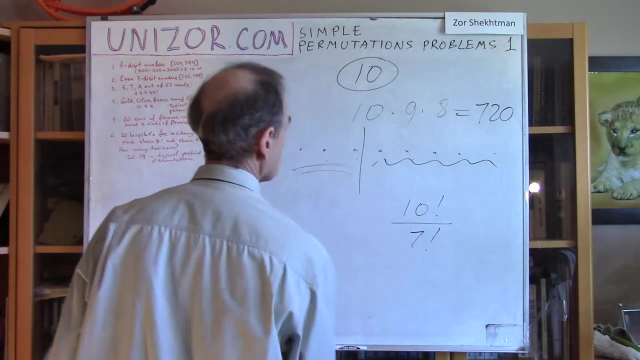 Product Of All Numbers, From Ten To One, And This Is From Seven To One, So Whatever Is Reduced, And Ten, Nine And Eight, So That's. 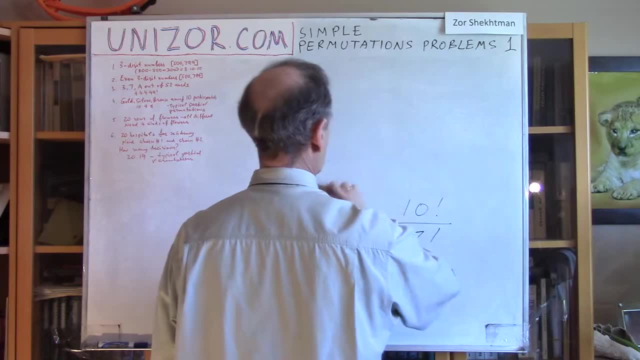 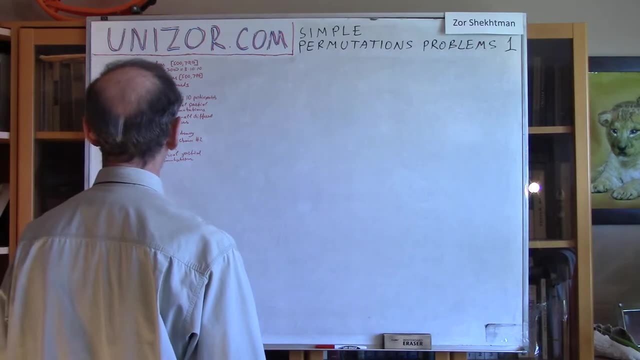 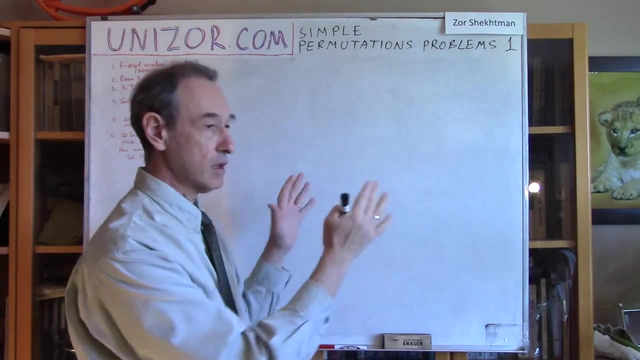 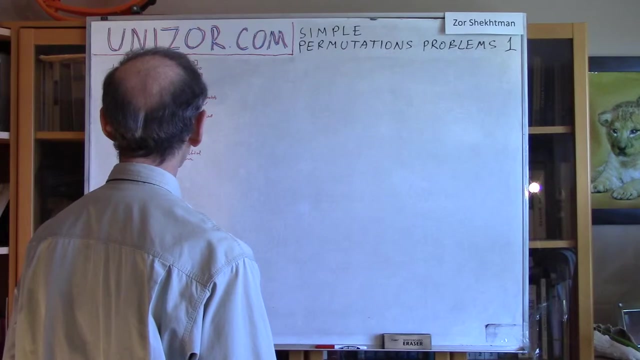 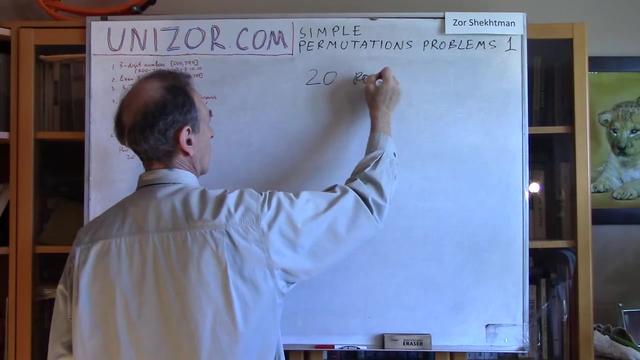 The Answer Next: Oh Yes, By The Way, This Is A Typical Example Of Partial Permutations, Because We Are Of Flowers. Okay, So You Are. 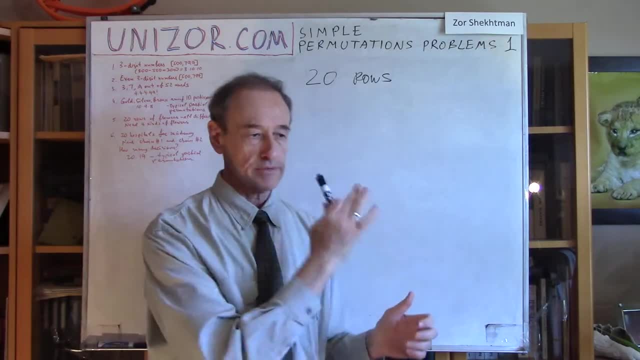 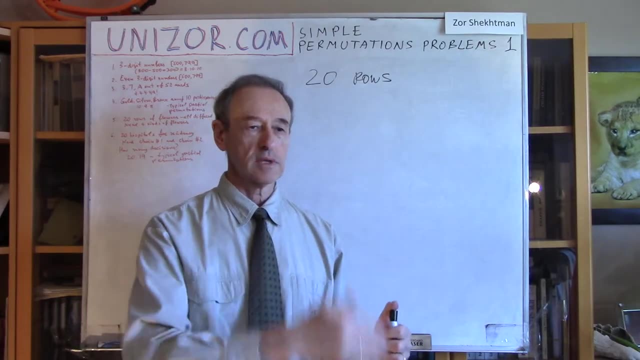 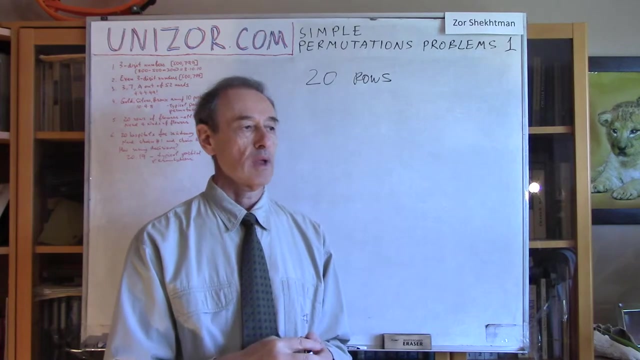 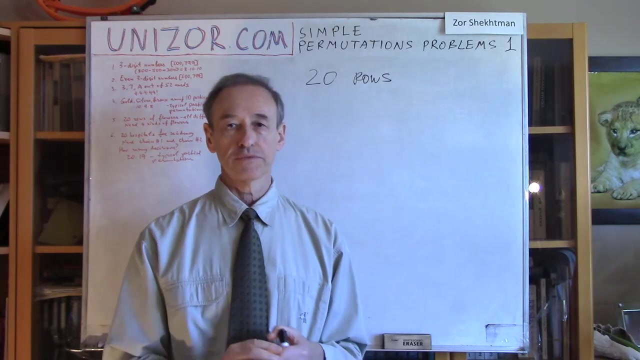 A Gardener And You Have Twenty Different Rows Where You Have To Put Flowers. Your Task Is To Put The Same Number Of Flowers To. 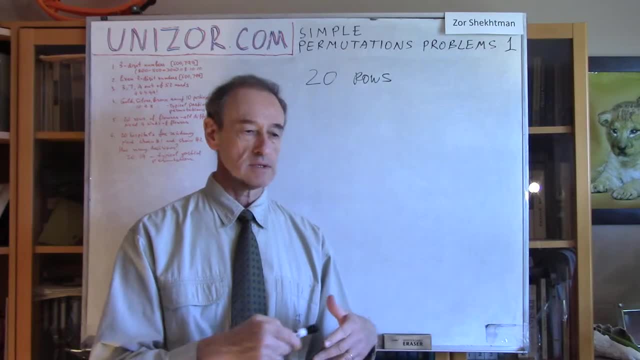 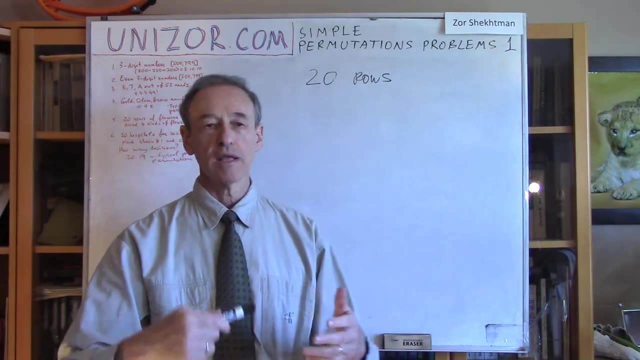 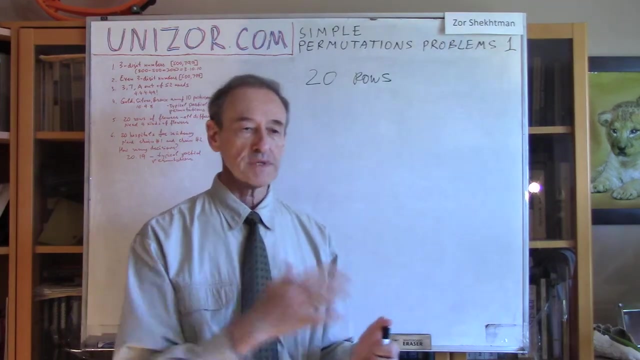 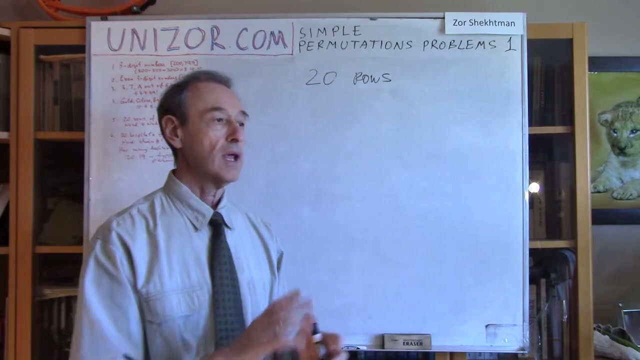 Have All Rows Different. So If One Row Contains Flowers Like A, B, C, D, E, Another Flow In Another Row Should Contain These Numbers. These Flowers, Types Of Flowers, Bushes Or Whatever You Call, How Many Types Of Flowers You Should Buy To Satisfy This Demand? Well, Let's. 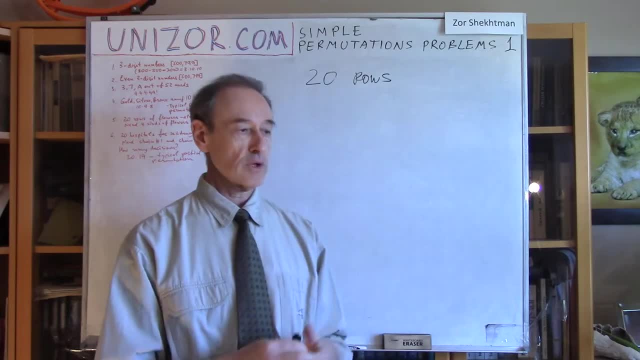 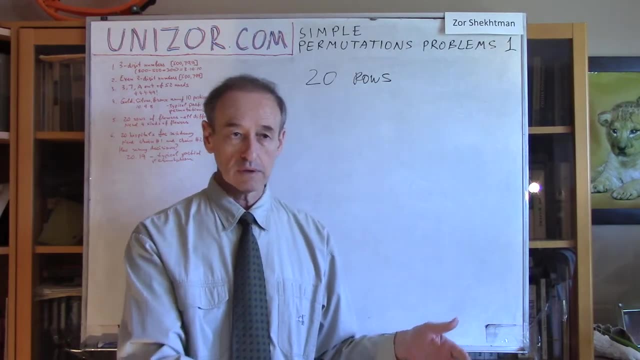 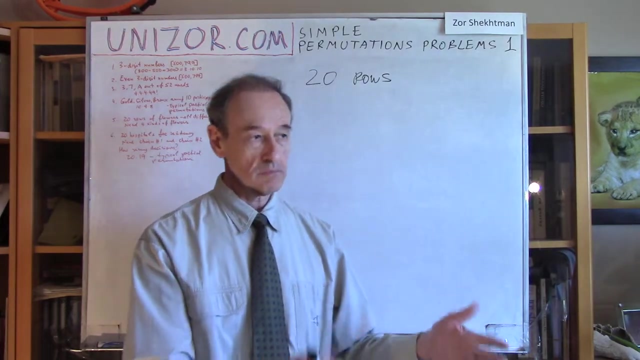 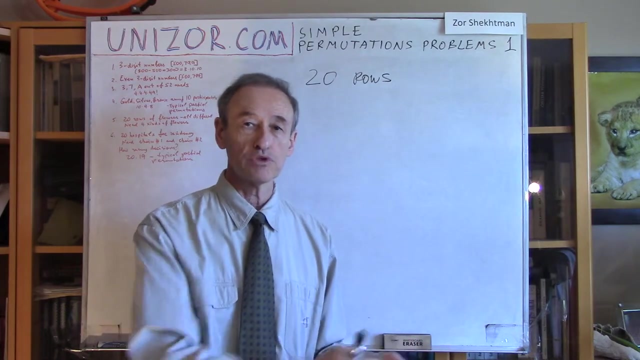 Just Consider: One Is One Sufficient. No One Is A Different From The Second Row. Now You Would Like The Second Row To Be Different. 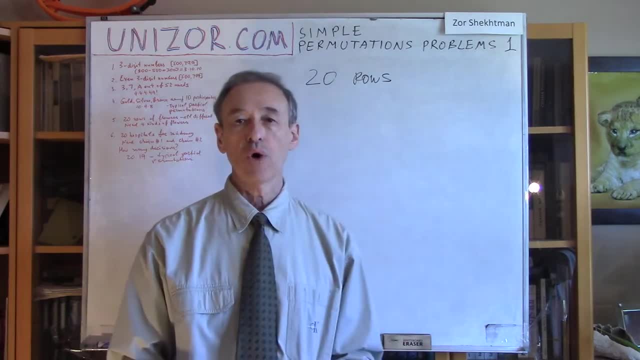 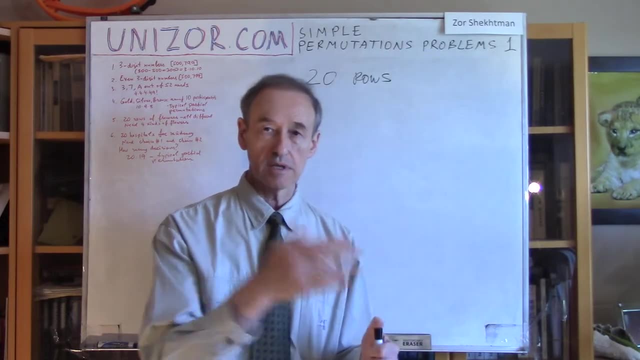 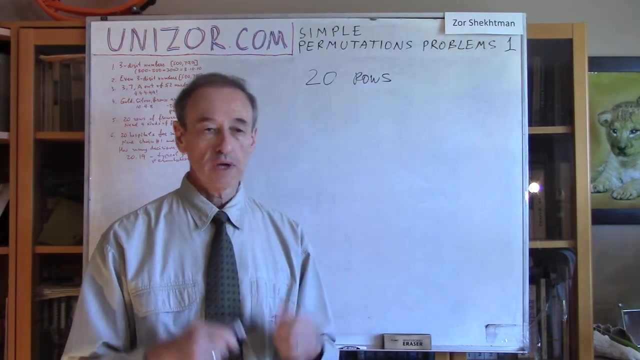 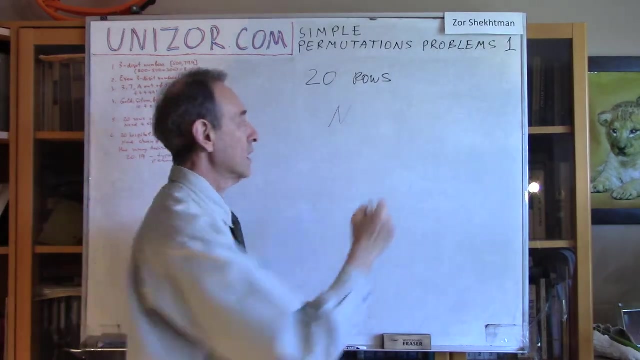 So You Can Probably Put The Second Type In The First Rows Different. Well, Let's Just Think About It Is Really Simple. If You Have, 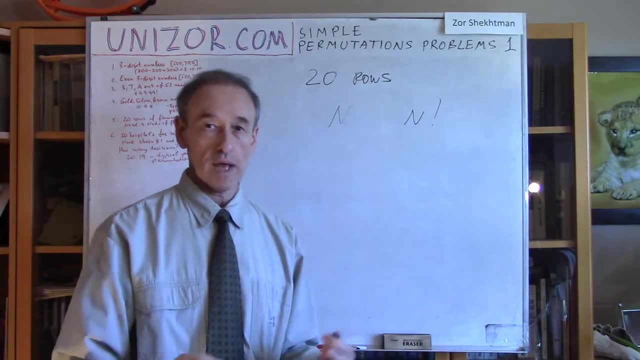 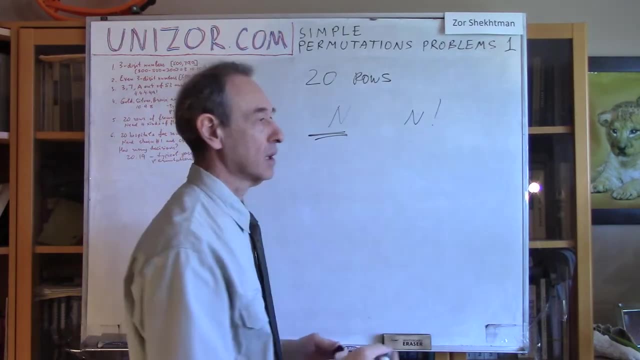 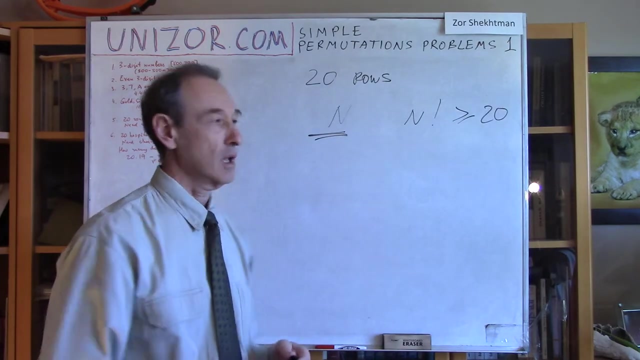 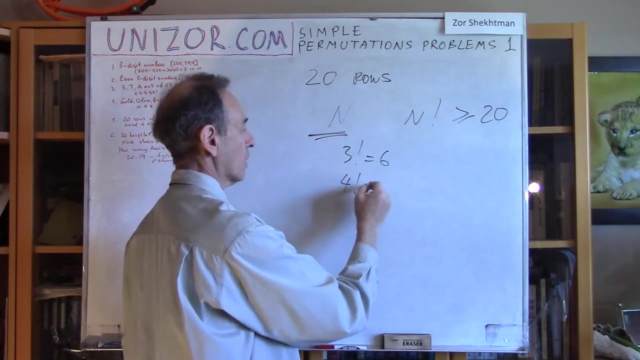 N Flow Different Types Of Flowers And Different Types Of Flowers. You Can Position Them In Different Orders, Which Is Sufficient To To Make 20.. 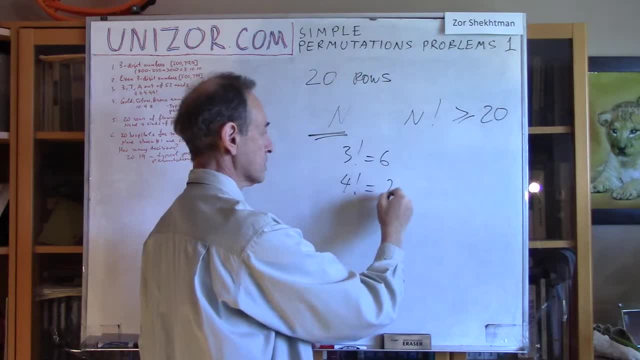 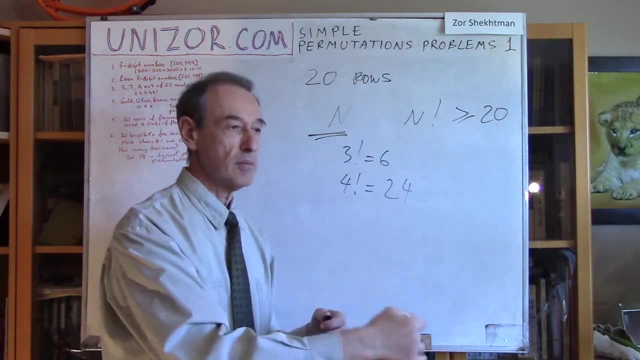 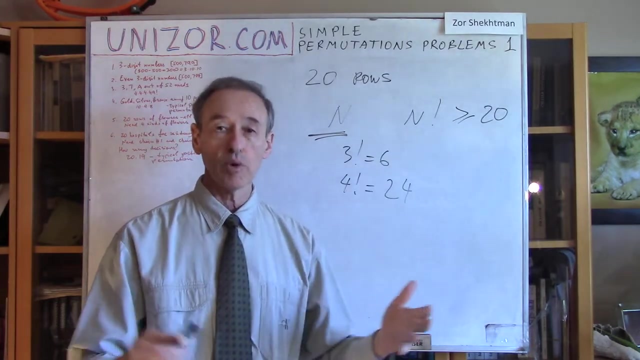 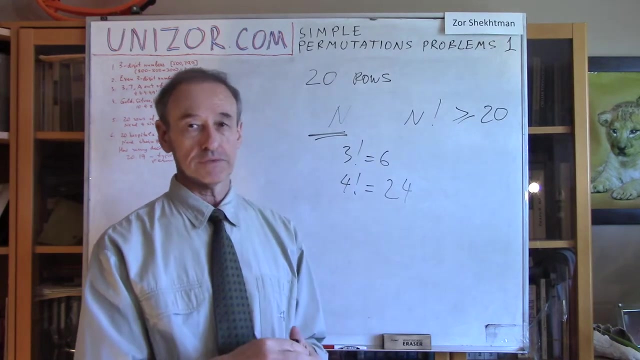 Rows Of Four Flowers So You Can Position Them In Different Orders, And There Are 24.. Different Orders, Which Is For Flowers Each Of Four. 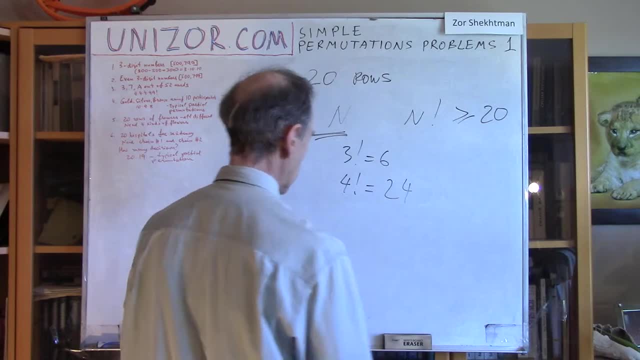 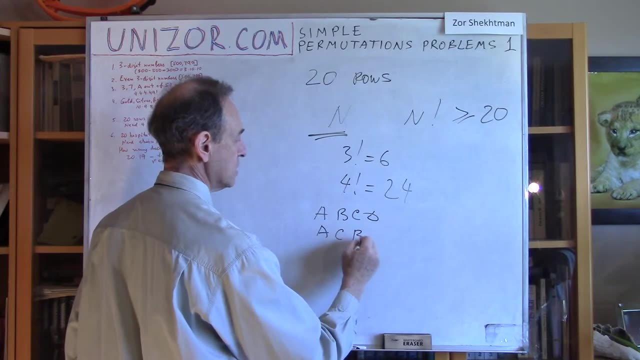 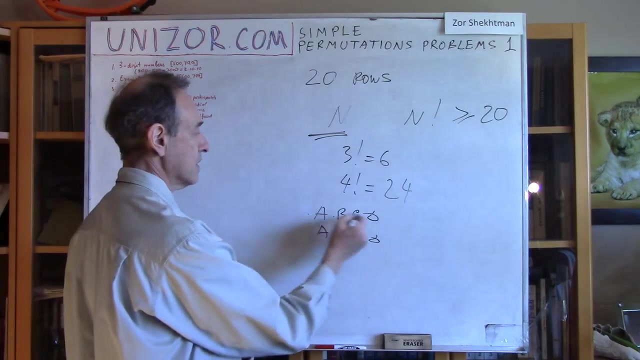 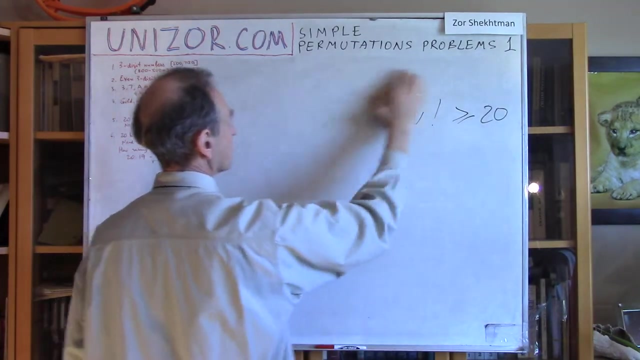 Types Of Flowers, Each To Make Them All Different. All Right, So Basically What I'm Talking About, You Have A, B, C, D, You, So 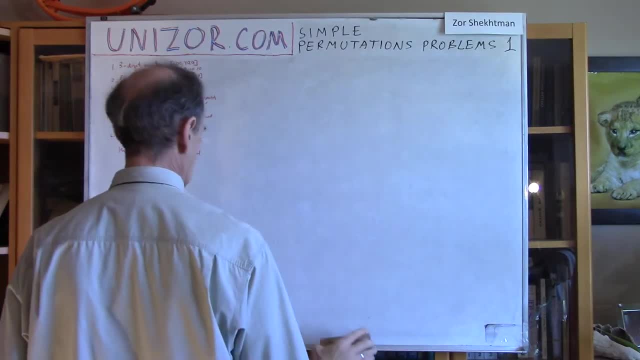 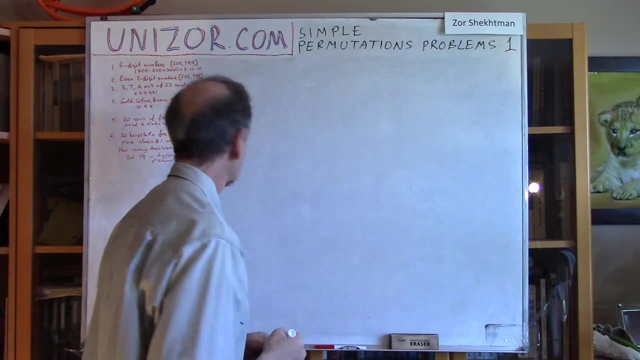 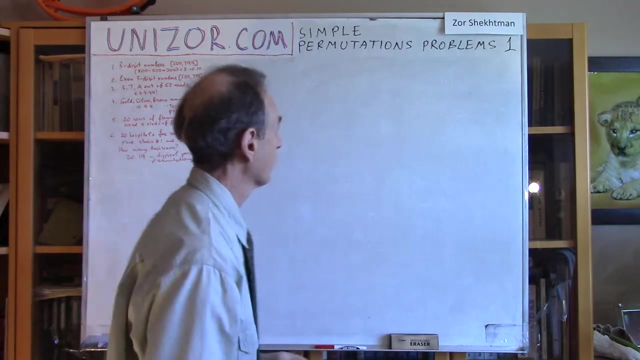 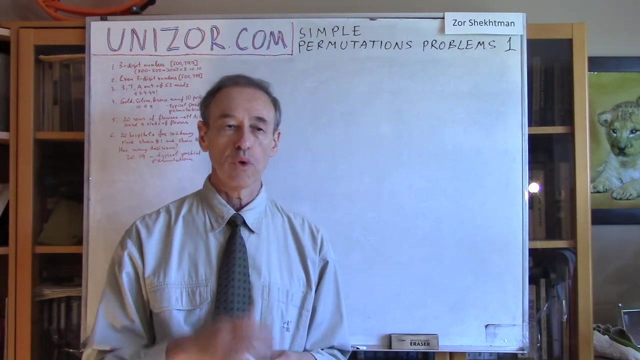 The Answer Is Four. Okay, Okay, It's Another Typical Partial Permutation Problem. Let's Say You're Graduating From The Med School And You Have 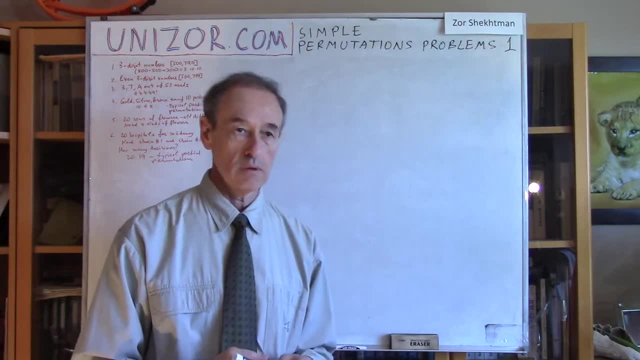 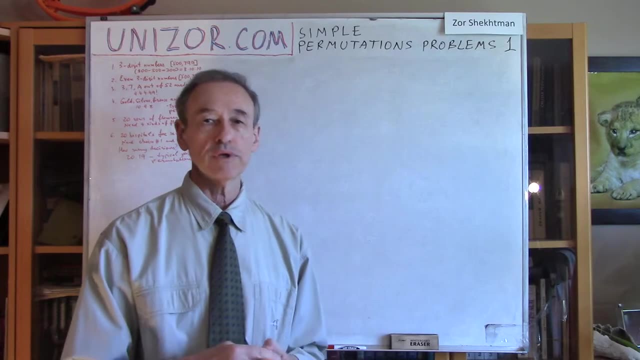 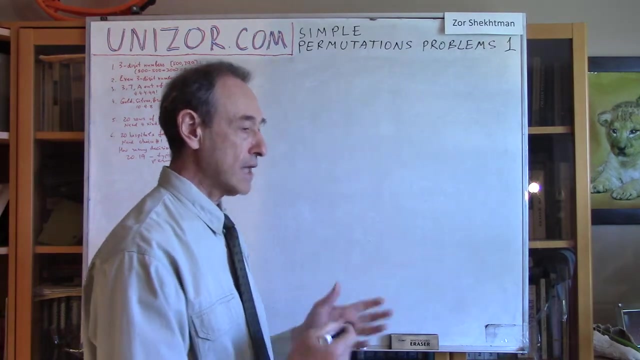 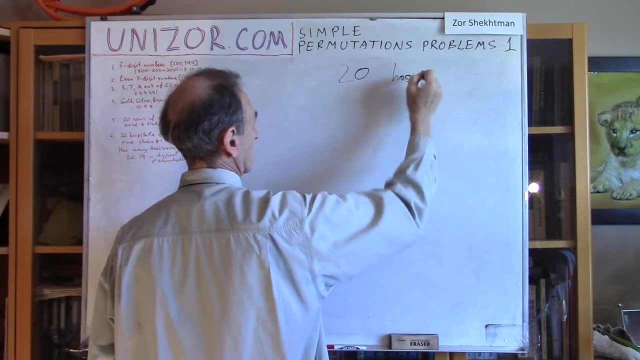 To Find A Place. Now, Let's Assume There Is Certain Agency. You Submit Your Documents To This Agency And They Are Helping You To Find. 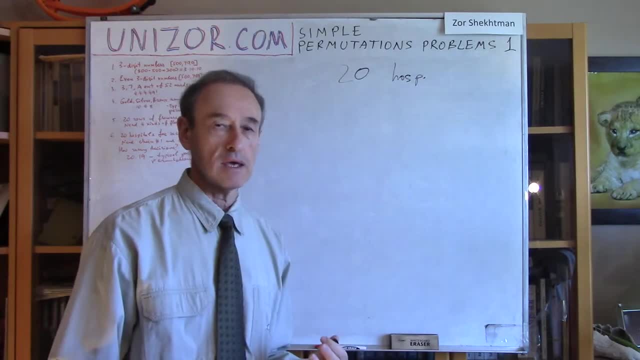 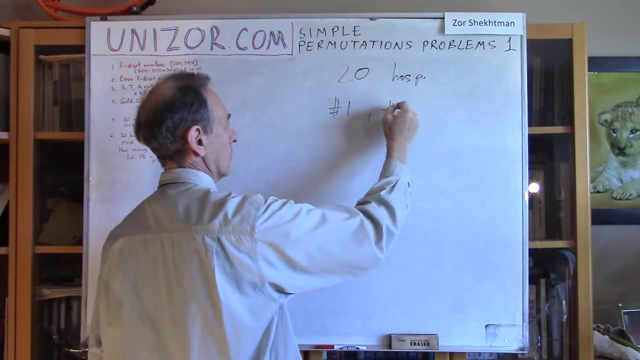 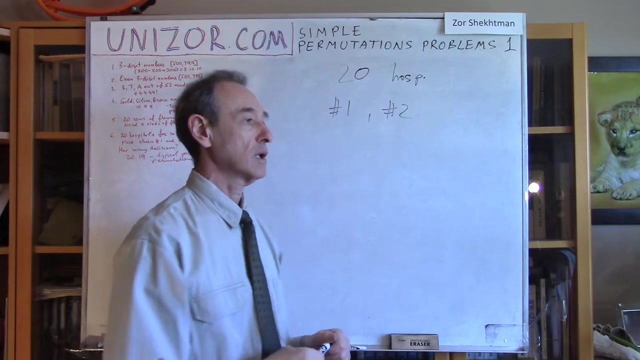 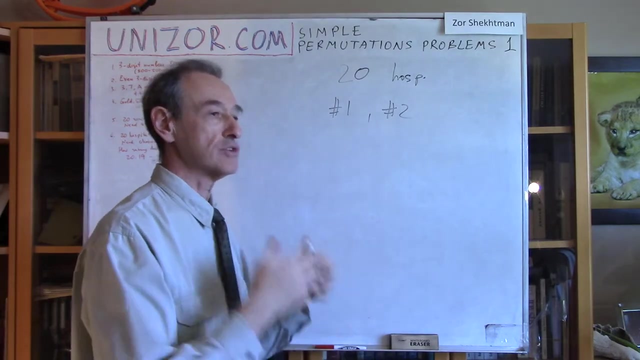 The Place For Your Residency, Number One Hospital, Your Choice, And Which Is Your Number Two Hospital. So You Have To Make Two Main Choices: 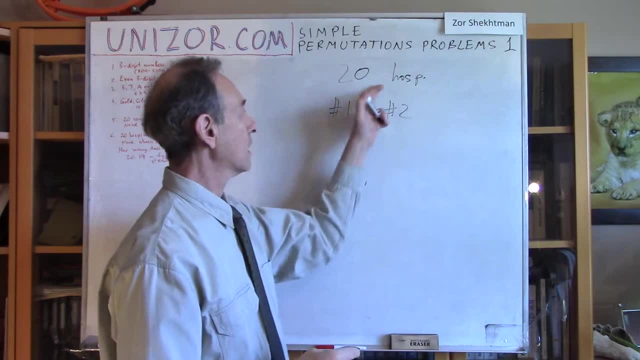 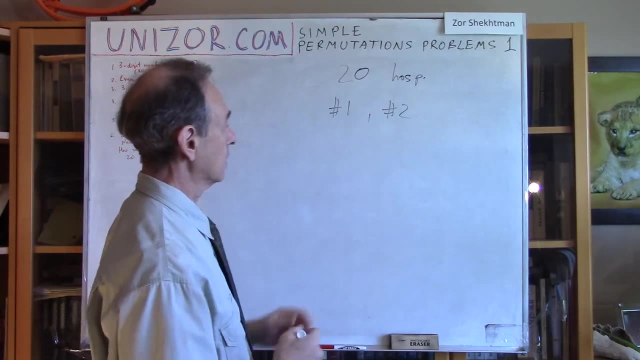 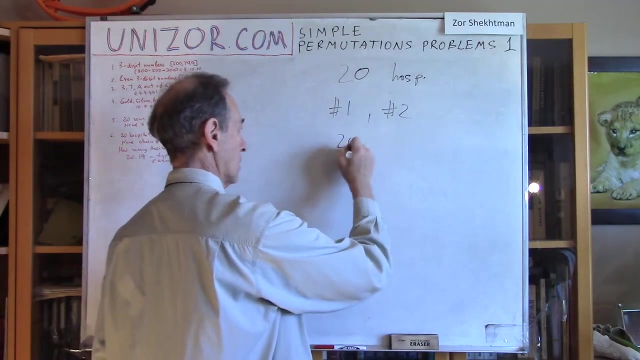 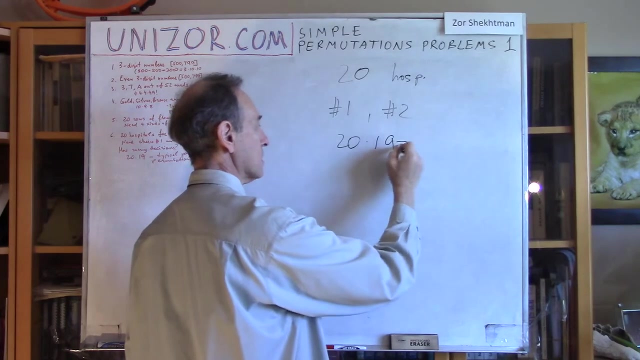 Now The Question Is Obviously, How Many Different Partial, And Again, The Typical Logical Consideration Is: For The Hospital Number One, You Have Twenty Different. 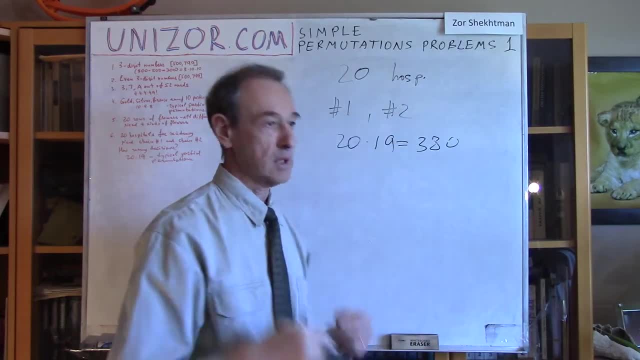 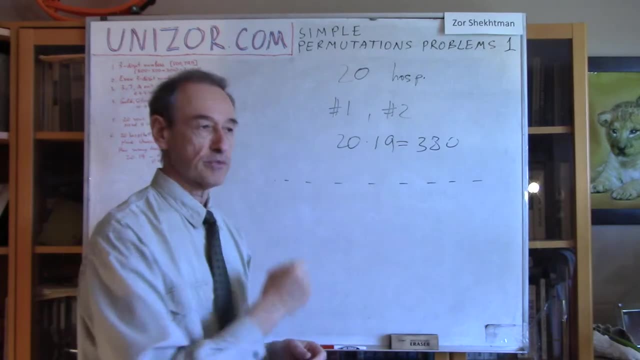 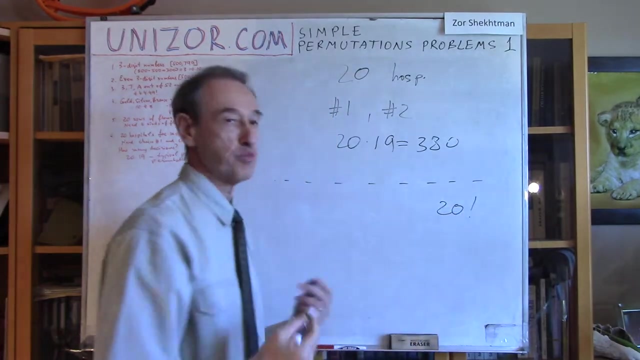 Choices, And For The Hospital Number Two You Have Obviously Nineteen Different Choices. Now There Are Twenty Factorial Different Ways Of Putting My Twenty. 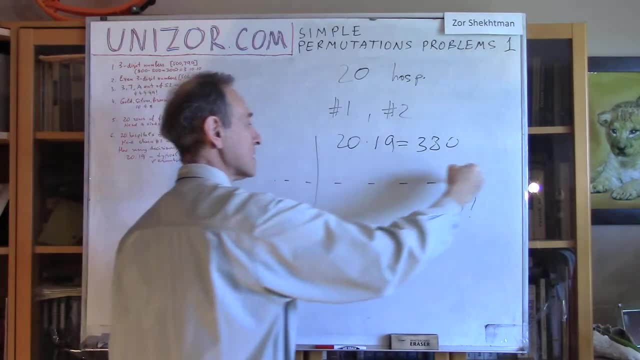 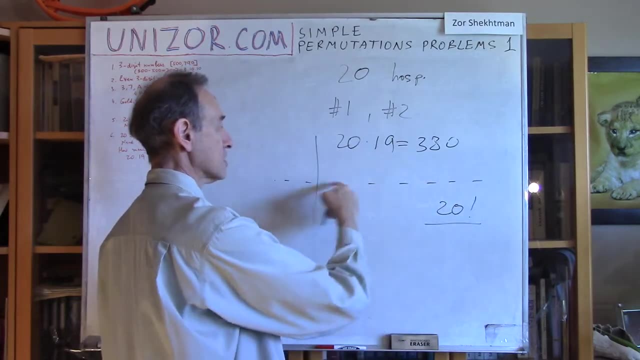 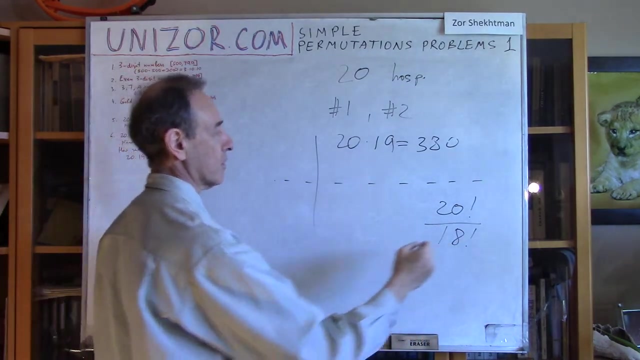 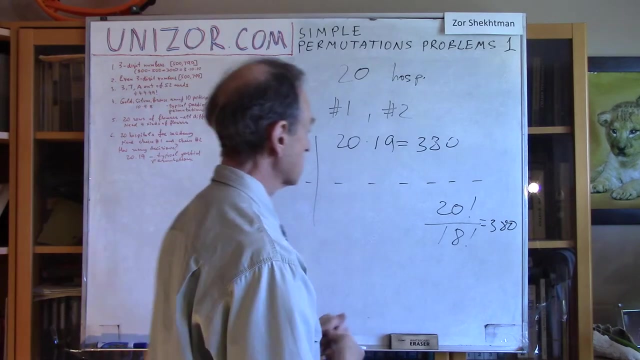 Hospitals In Some Order, And I Cut The First Two, This Is Number One, This Is Number Two. Three, And The Number And Number Of Permutations. 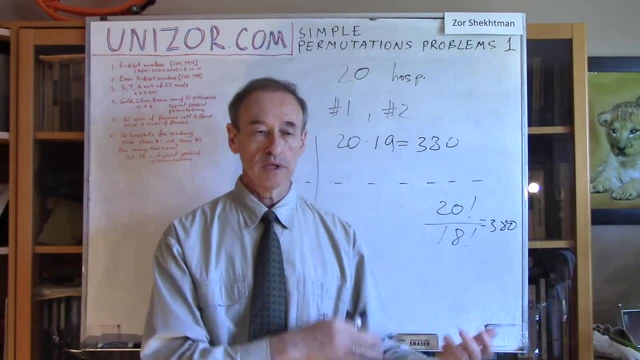 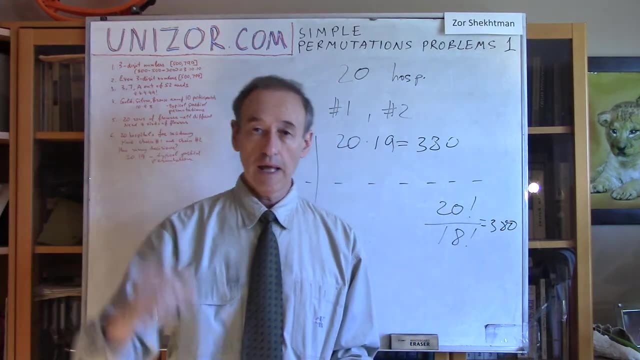 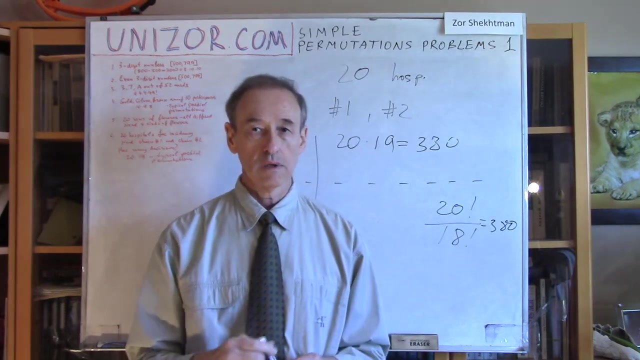 I'm Looking For. So That's The Result, And This Is My Last Problem. What I Would Suggest If You Didn't Do, Come Up With.